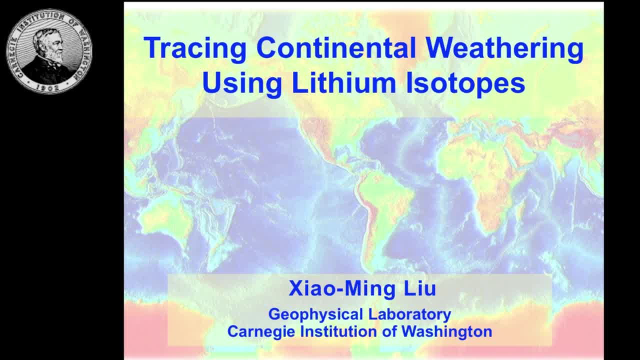 So today she'll be talking to us about tracing continental weathering using lithium isotopes, and I'll let you take her away. Yeah, thank you, Lara, for this very nice introduction. Thank you everyone for coming. Okay, so let's just start it. 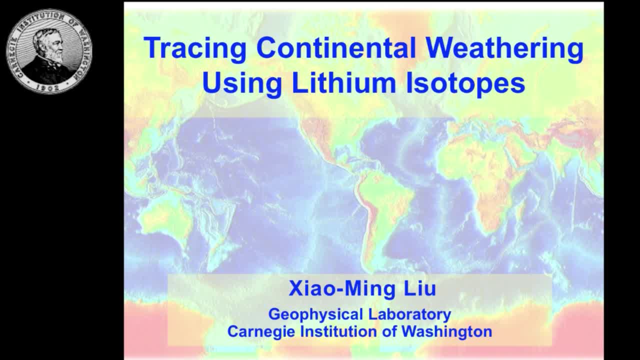 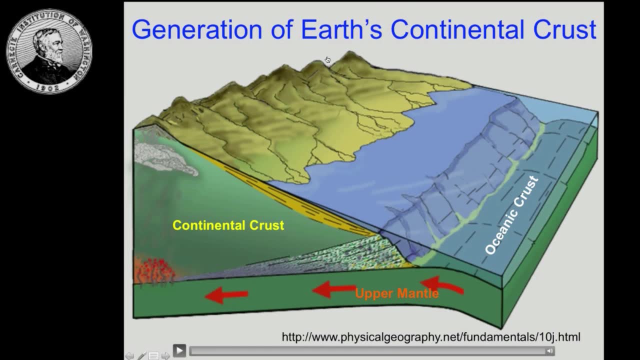 So today I would like to talk to you about using my favorite isotopic system, lithium isotope, to study continental weathering. Okay, let's start. first, Let me show you a very nice cartoon about how the continental crust is generated. now 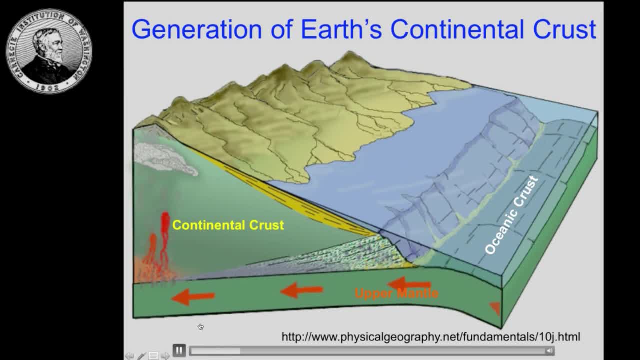 We see that the continental crust is generated. It's usually generated at the arc settings, where the existing continental crust is colliding with oceanic crust, and then we have melt generated. Then we have either eruption of volcanoes or plutonic intrusions generating the new continental crust. 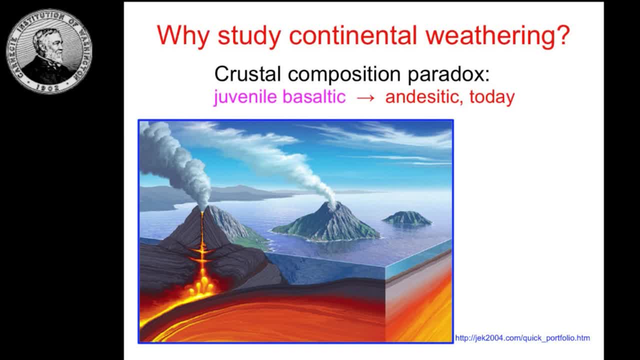 So why do we care about continental weathering? right, There is a so-called crustal composition paradox. We know that the magma that generated the current day continental crust is basaltic. At least the majority is at these convergent margins. However, the subalcanal crust, the one that I'm standing on, that you are sitting on today, is antacetic in composition. 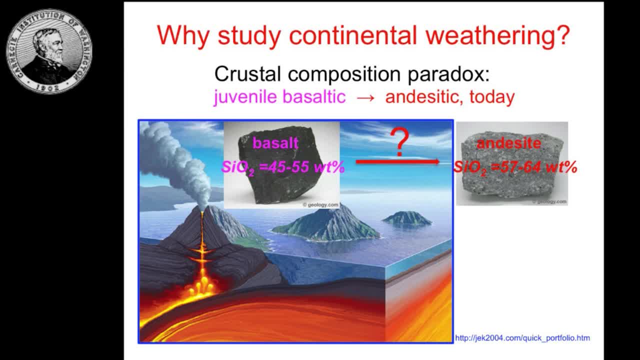 So I'll just show you what a typical basalt looks like- a rock basalt, and the underside looks like. So they are actually different in terms of silicon content, right? So the more we call it more felsic, it's more silicon-enriched. 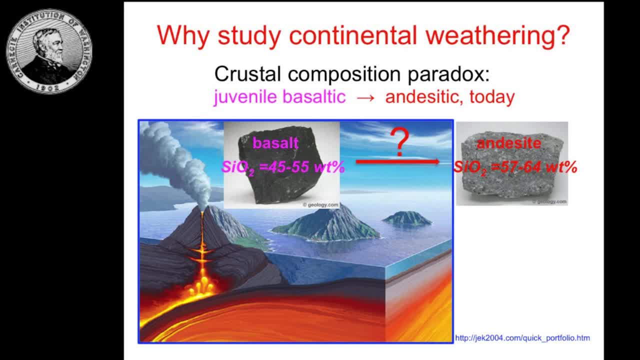 More mafic, meaning more basaltic composition. So this is the discrepancy between the building block and the building right. It's usually referred to as crustal composition paradox. So many hypotheses have been proposed to solve this crustal composition paradox. 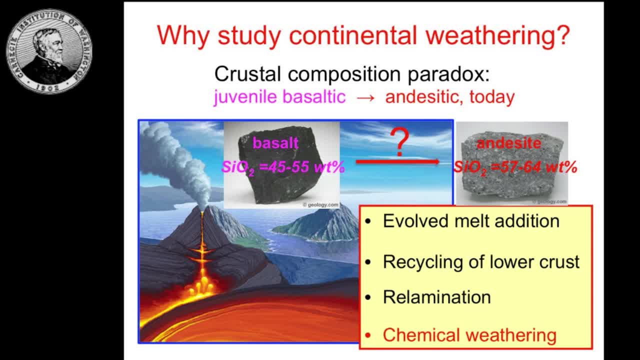 including involved melt addition in a hot racking, because the racking may have a higher degree of partial melting. We have more felsic crust at that time, So the dual crust may be not entirely basaltic as it is today. Also, there is an idea of recycling of the lower ultramafic and mafic lower crust. 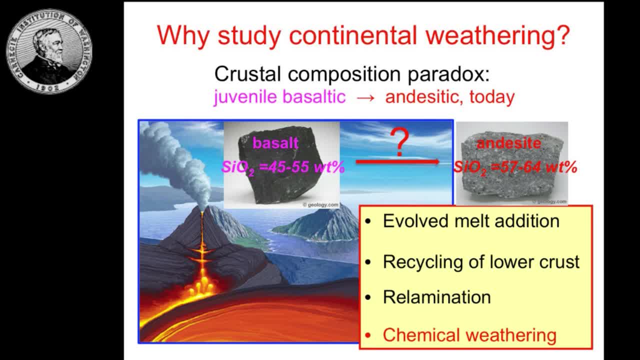 because the lower crust is more mafic in composition. So by detaching from the components we get the bulk crust to be more antacetic. And also there is a new idea of re-lamination followed by subduction of more felsic crust onto the components. 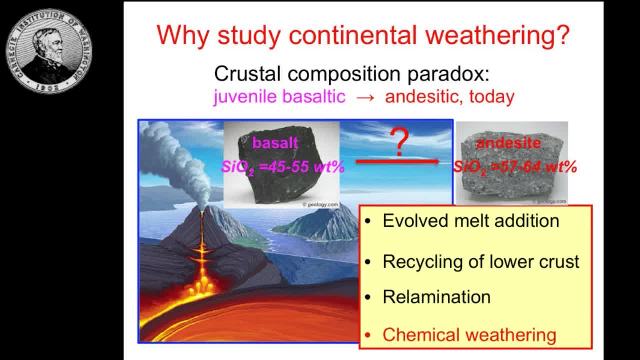 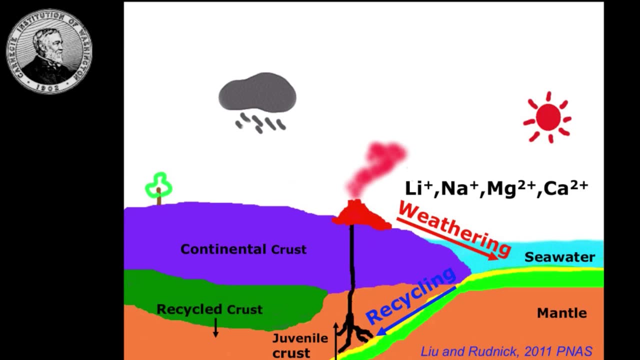 So we could have more felsic crust that way And, of course, the focus of today's talk. I'm not going to talk about three other mechanisms. I would like to pay more attention to chemical weathering as one mechanism to changing the crustal composition and mass. 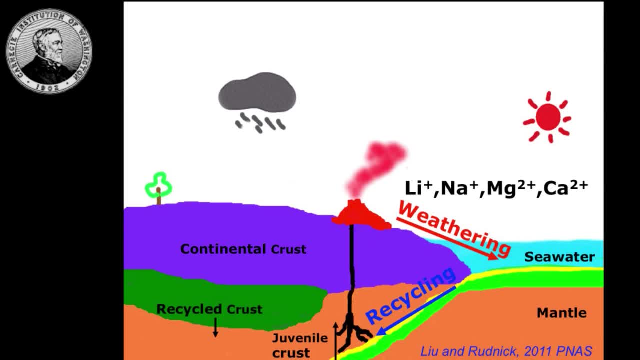 So this is a very childish cartoon. I do it So it's not to scale, of course, Okay, but this one just gave you an idea of what I'm talking about, about chemical weathering. Chemical weathering preferentially removes soluble elements. 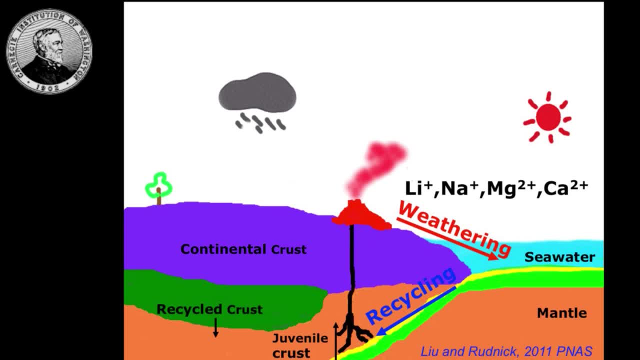 such as lithium, sodium, magnesium and calcium and removes them into the oceans, So that leaves the continental crust to be more silicate-rich. So that's one possible mechanism. However, traditionally in the high-temperature geochemistry community people think this is not an important mechanism. 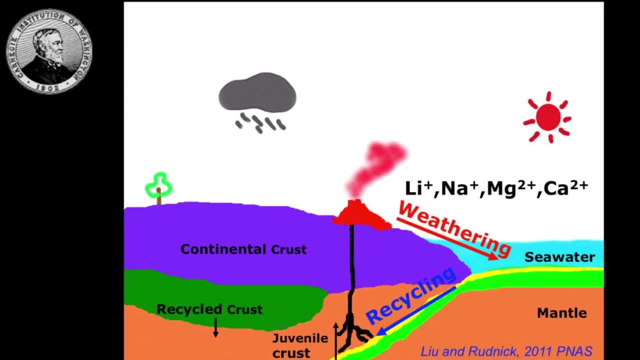 because this is only a top-down process, right? It's only up to the upper crust, a couple hundred meters distance, right? However, how important is important, right? We need a way to quantify. So we did a. Steve is not here, I guess. 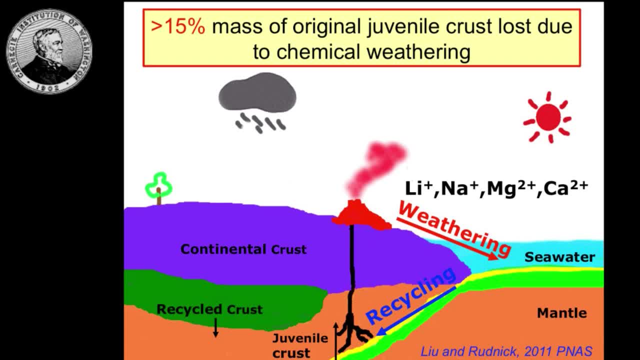 But I don't want to put the rest of you into sleep So I don't show you the mass balance model. So we actually did a mass balance model based on lithium isotope to look at the input of the continental crust and the output to quantify how much of the mass is lost due to chemical weathering. 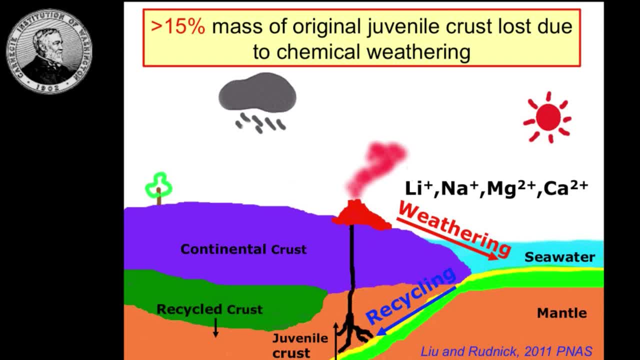 from the dew in our crust. So I'm not going to show you the mass balance. You can check our papers a couple years ago And you just have to believe me. It's important because it's 15%. It's our minimum estimate. 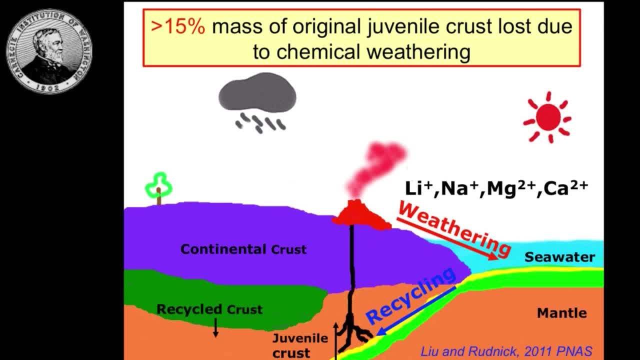 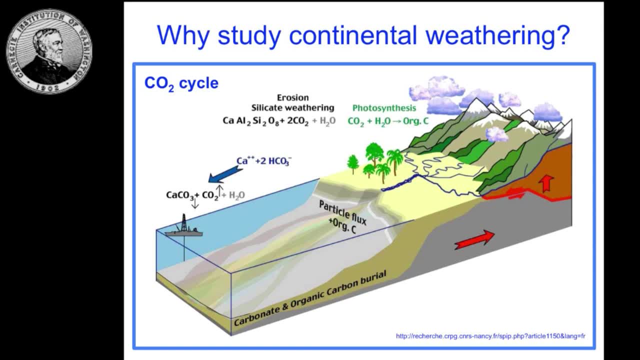 So that's another motivation. That's another motivation why we need to care about continental weathering right. Okay, Another important reason is we know that tectonic uplift is increasing the continental erosion right And also continental weathering, especially continental silicate weathering. 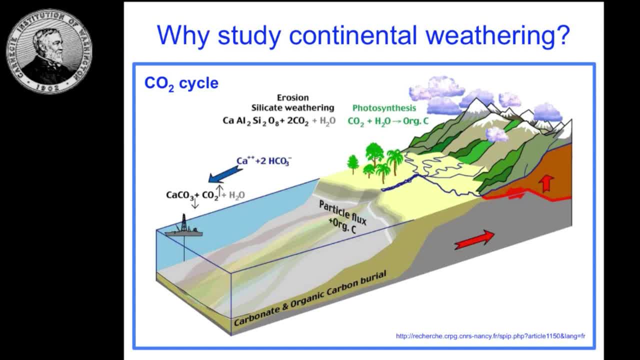 is the net output for the CO2 in the atmosphere. As you all know, the CO2 is important in terms of regulating the climate, at least in this geological scale we are talking about. We're not talking about the future climate change, Anyway. so continental weathering is actually a natural connection. 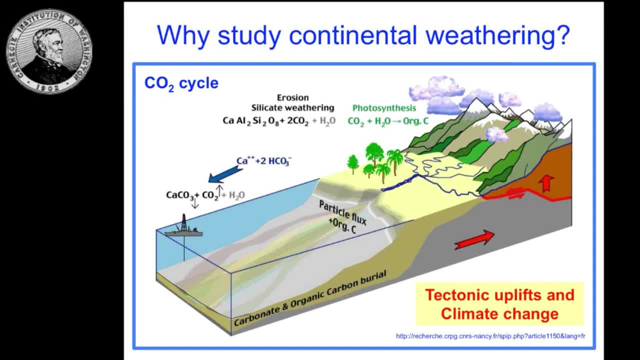 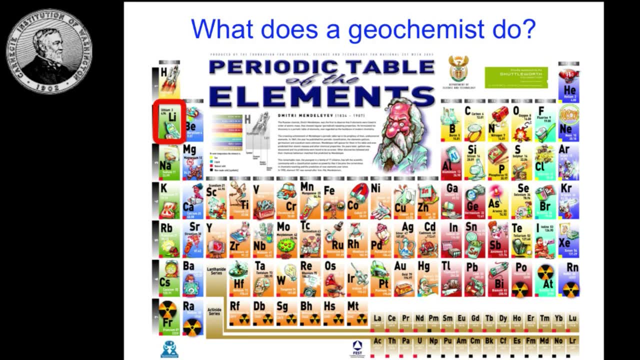 for the tectonics and also the climate change, So it's an important link we need to investigate more. Okay, so I'm a geochemist. I like to look at the periodic tables every day And we want to find the best system to study the geological processes. 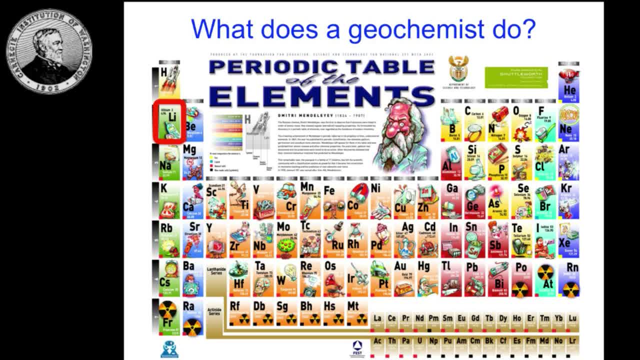 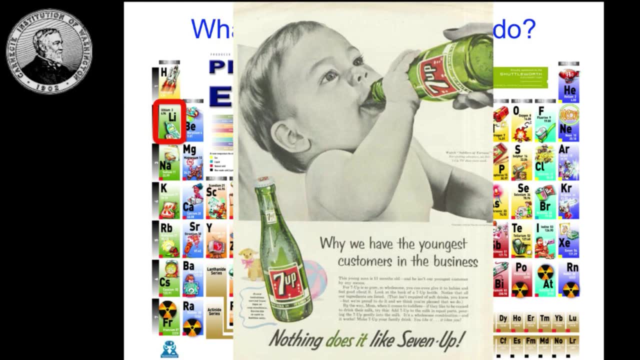 we want to study. In our case it's continental weathering. So lithium is great in terms of continental weathering, not only because it's important in our laptop and phones as the batteries, but also this: Have you drink this very interesting drink, 7-Up? 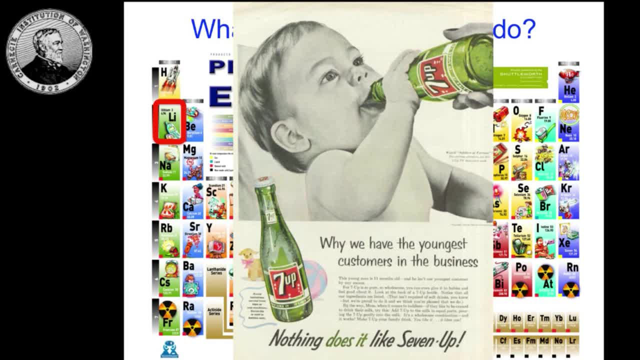 This is probably the very first commercial of the 7-Up, So I actually speculate why this drink is called 7-Up, You know, before 1950s. they add lithium citric in the 7-Up, And lithium is a known modulating drug. 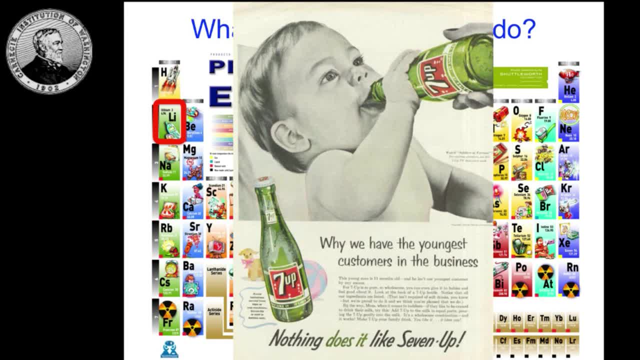 Actually nowadays we take lithium to treat bipolar disorders etc. So it can potentially make you happy, as this commercial says. So nothing does it like 7-Up. I was a happy baby. Probably people who grew up before 1950s are happier than us. 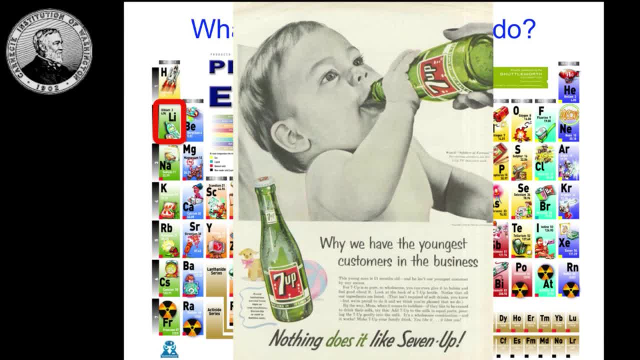 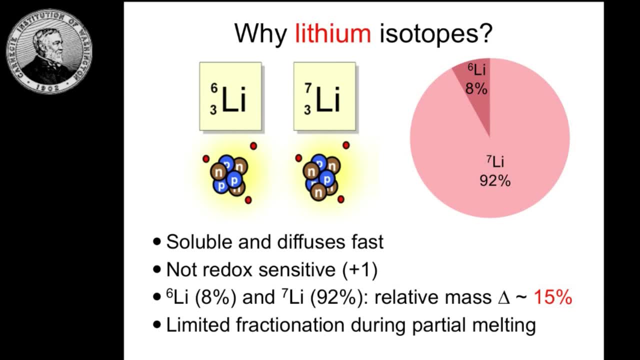 Now we don't have this good stuff in there, Okay, so if being happy is not enough reason, we have more reasons for using lithium. Lithium has two stable isotopes, lithium-6 and lithium-7.. As you see, the 7 is more than 90%. 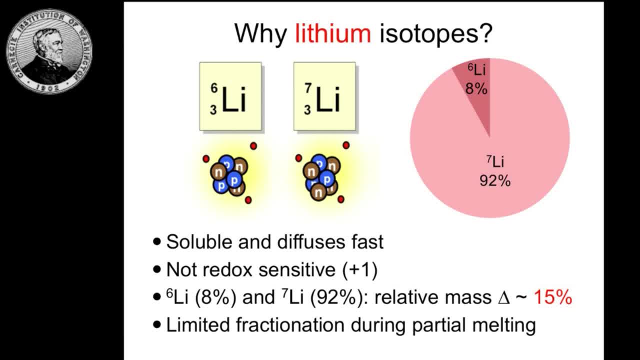 It's a majority. Lithium diffuses really fast and also lithium is soluble, So it makes it very well in terms of transportation process during fluid-rack interaction And also because lithium has only one redox state so it doesn't get into very complex redox reactions. 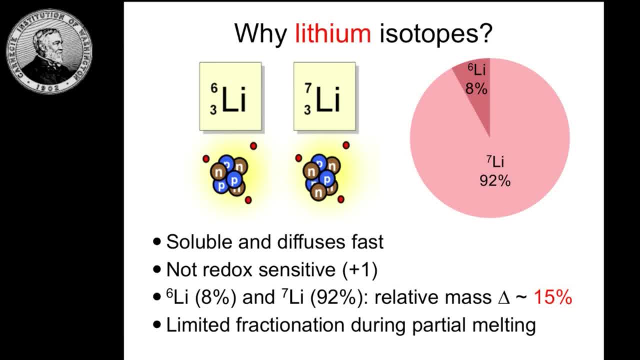 which is good in terms of weathering processes. As you already noticed probably, lithium has a very light element. Therefore the two isotopes- 6 and 7, has a relatively large mass difference between 6 and 7. So it can give rise to very large isotopic fractionation potentials. 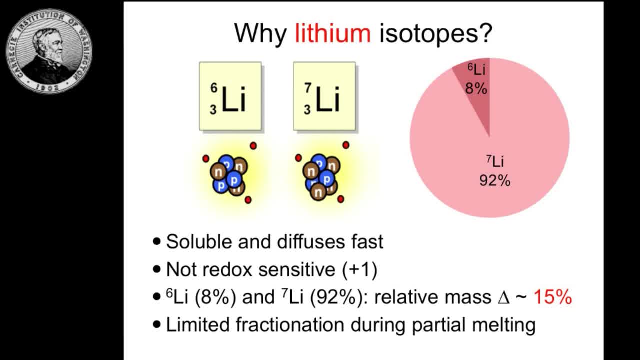 the mass-dependent fractionation And also the also bonus point is we know that lithium has relatively limited fractionation in high-temperature processes such as mantle partial melting, So it's great for tracing low-temperature fluid-rack interactions such as weathering. 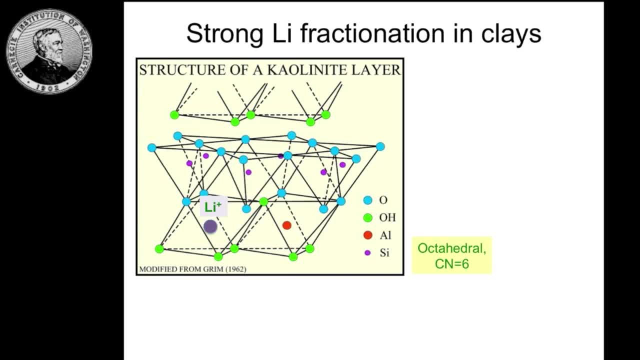 Okay, so this one shows you a diagram of what a typical product weathering a clay mirror looks like. So this is a kaolinite mineral structure. Lithium likes to replace the aluminum in the octahedral structure. Versus in waters, lithium likes to bond. 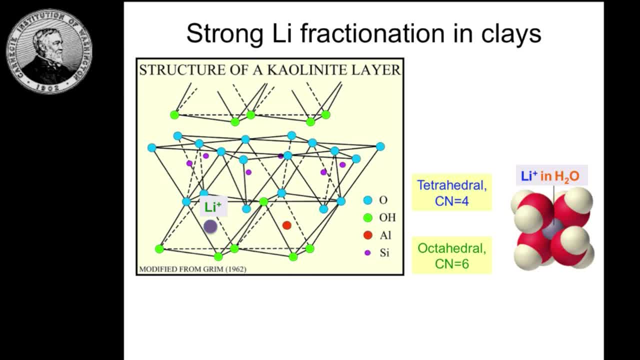 with four different water molecules to form this tetrahedral structure. So this is actually known. from very fractionation mechanism theory that we know, the heavy isotope prefers the higher bonding isotope in the octahedral site and usually corresponds to low co-ordination number. 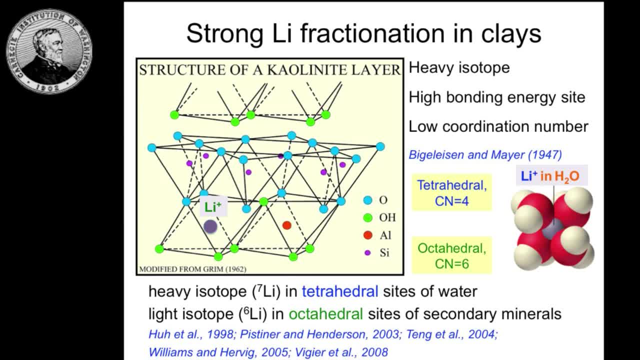 So that means the heavy lithium likes to go into the tetrahedrally co-ordinated water, and then the light isotope likes to be in the octahedral site of the secondary main earth, such as a clay or iron-aluminum hydroxides. 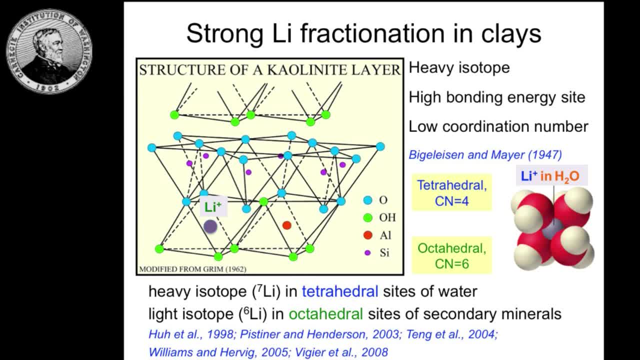 This has been well established by many observations as well as laboratory experiments. So that's the fundamental fractionation we will use in tracing weathering processes. Oh, by the way, if you have any questions, you can ask in the middle. Okay, hopefully by now you're so excited. 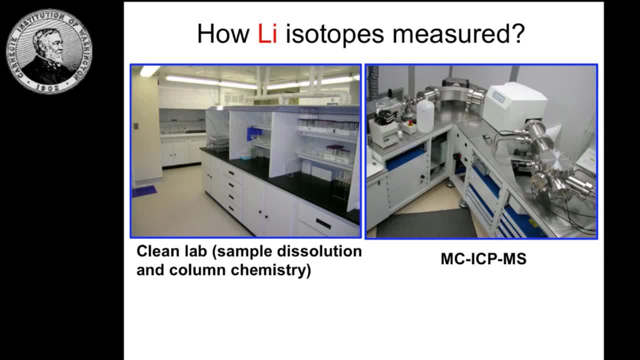 you want to know how do we do it right? How do we measure lithium in the laboratory right? As a geochemist, we work with geologists also. some of us are geologists, So we go out, we pick up the samples. 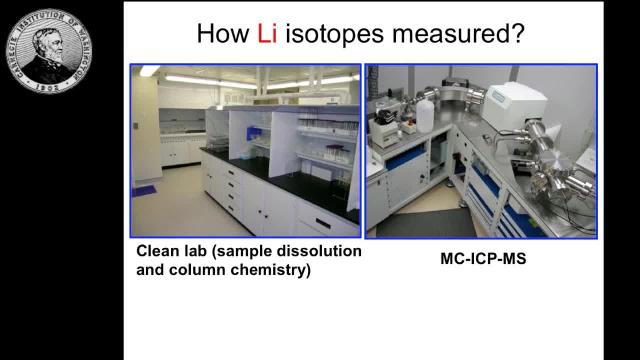 either in forms of rock or water, and then we for the rocks, we cut them into powders in the end, and water, we evaporate the water, the majority, and then leaving the lithium in the solution. So then we do laboratory experiments. 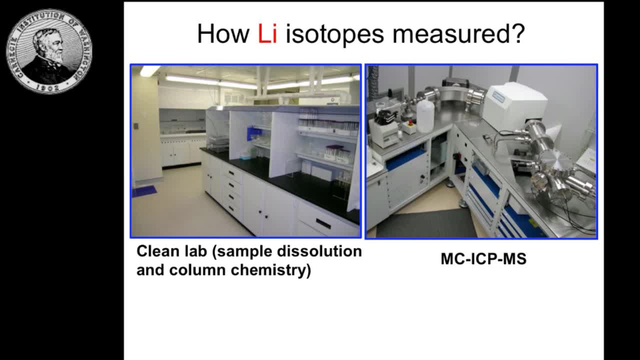 for sample dissolution, where we use very strong acids like hydrofluoric, hydrochloric and all the very dangerous acids to dissolve the rock or water sample- anything you want, basically- And then we can go through for isotopic study. 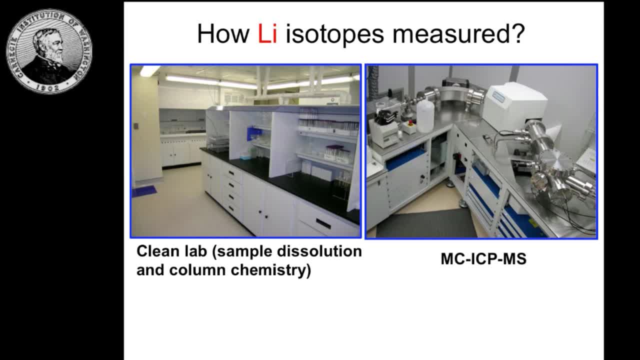 we need to purify the solution because we only want the isotopic system of interest, in this case lithium. So we set up a chemical exchange called autography to get rid of other elements that we don't want, But basically we only have lithium solutions in the end. 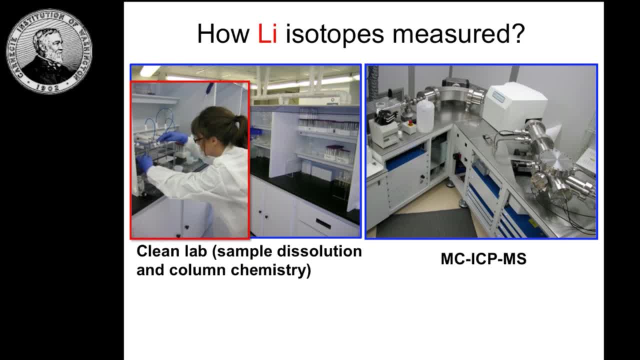 So this is a very laborious process, so it needs a lot of crying time in the lab, or happy time in case of lithium right. So we have then taken the purified solution into this multicollector ICP-MS, So it's a plasma source mass spectrometer. 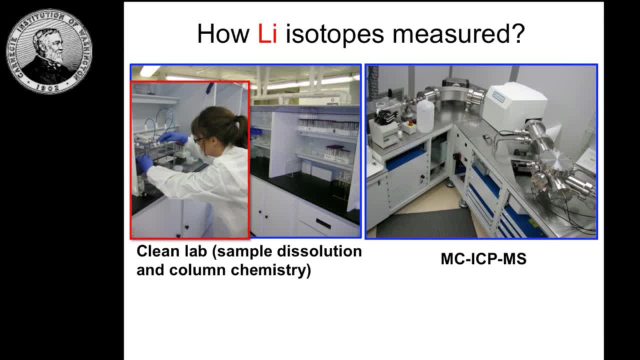 This is actually the closest thing I think on Earth you can get to the surface of the sun, because the plasma temperature is 8,000 degrees C up to. So you basically at that temperature you can ionize everything. So we put through the purified lithium solution. 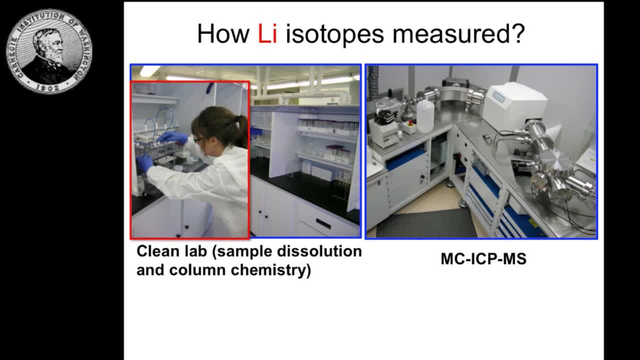 go through electrostatic analyzer and then the big magnet where you can separate two isotopes- lithium-6 and 7, in terms of their mass difference, And then at the end it goes to a collector. It's actually basically big resistors. 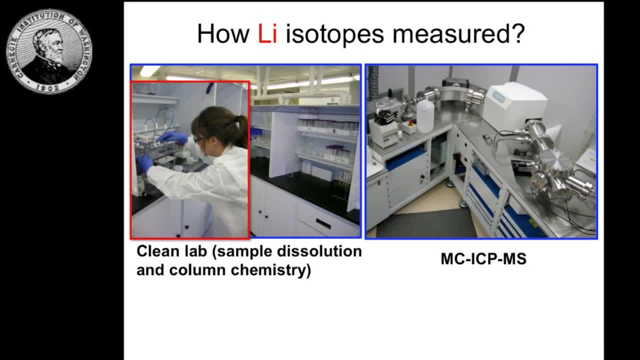 When you have current, hit the resistor then you get a voltage. really That's how we get the isotopic ratios. As other stable isotope systems like carbon and oxygen, we express isotopic fractionation using the standard delta notation. So it's lithium-6 to 7 in the samples. 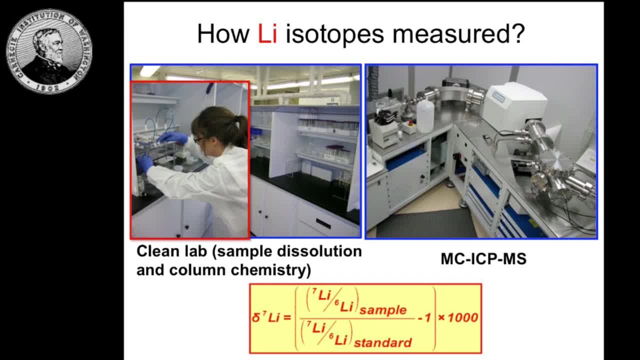 divided by the 6 to 7 ratio- Oh sorry, 7 to 6 ratio, Always heavy versus light- And subtract 1 times 1,000, so we can get a big number to work with, not .000, something right. 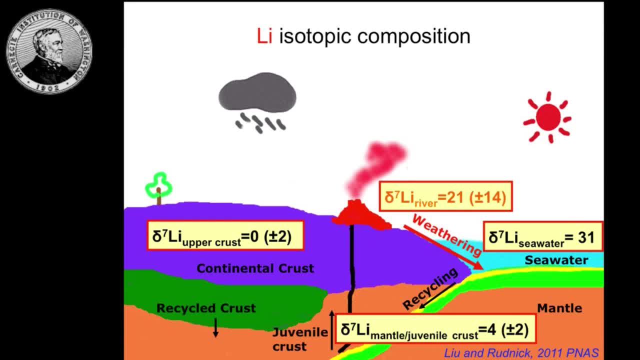 Okay, So now you're going back to this cartoon, We can see how delta lithium looks like in weathering-related research. We have a relatively homogeneous mantle composition. It's about 4 plus or minus 2.. The upper common cross is a little bit light. 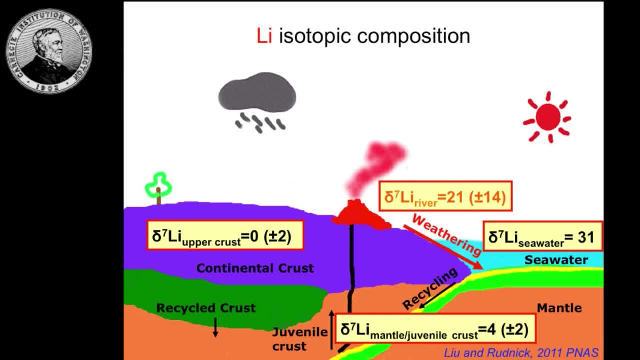 because the fractionation I told you before, right, The formation of secondary minerals like clays, prefers the light isotope. So the upper common cross, especially, has been through weathering. So we have the light values. And then I would like to point out the water. 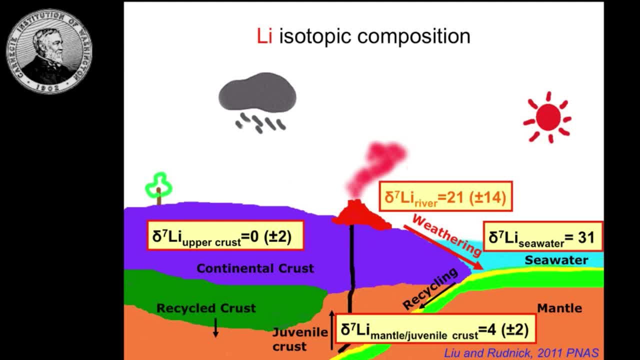 they interact with. the rock right Must have heavy value to make the mass balance work And the seawater additionally have even heavier value because there is additional oestrogenic clays formation on the seafloor so we have further fractionation from the rivers. 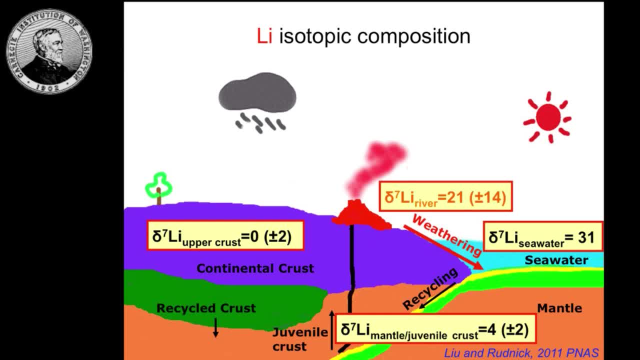 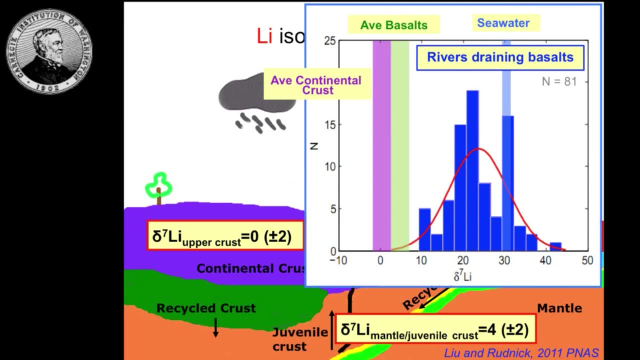 but that's not a topic I want to talk about now. So if you don't, If you haven't looked at this, I will show you a more pronounced histogram. The problem here is we have Average upper common cross very homogeneous. 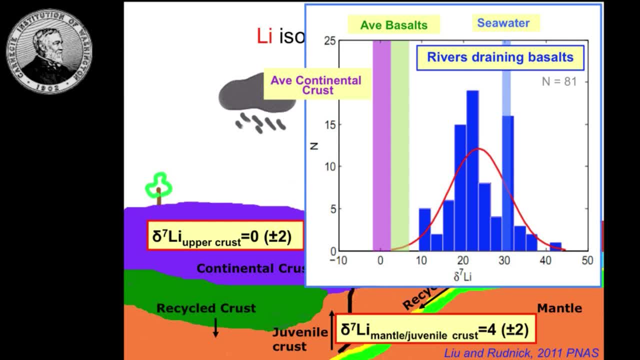 Average basalt relatively homogeneous. Oh boom, you see there is a huge variation for rivers that even only draining basalt, It's a single lithology of small rivers. They have like 30 per ml fractionation, right. 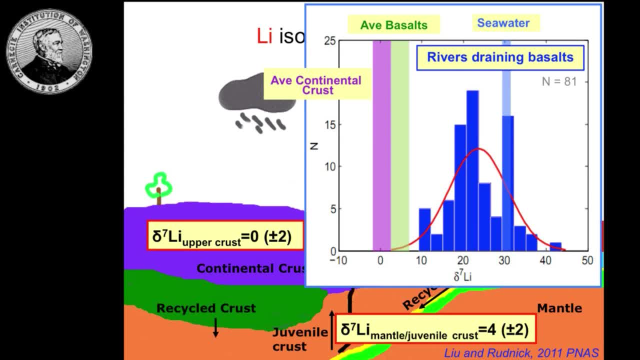 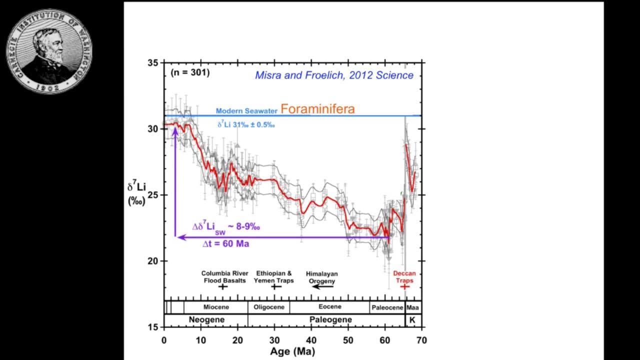 It's one of the big questions that motivates my study is what controls lithium isotopic fractionation during weathering, Why the rivers have such a wide variation in terms of isotopic composition. right So, And there is another one. There is a paper, interesting paper. 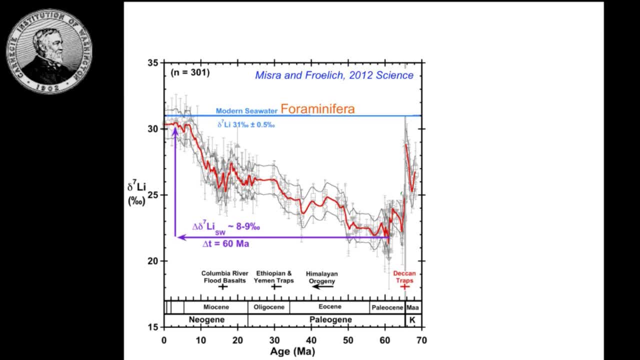 published a couple of years ago using foraphenifera- a cute fossil- as a paleo-oceanatic proxy to look at the lithium isotopic variation through time right. So basically what they found is through the synozoic there is a 8 to 9 per ml increase. 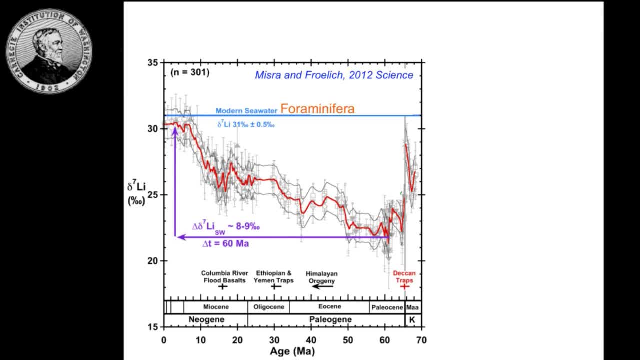 in terms of delta lithium from the synozoic to now. So what this means, right? So is that? Is that meaning we have more vaseline Because lithium is really low content, has really low content in the carbonates, right? 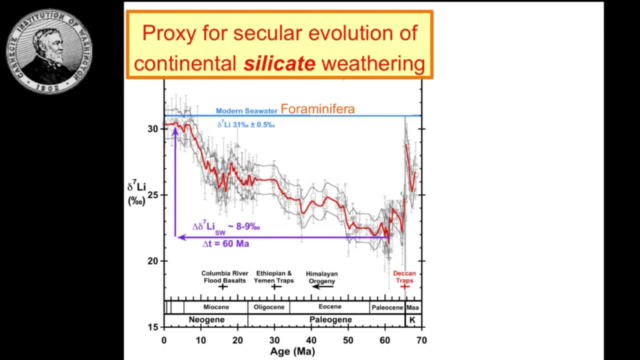 And it's very enriched in the silicates. So they're invoking a proxy for secular evolution of the content of silicate vaseline, especially because lithium is not much in the carbonate. However, if we consider a mass balance in current seawater, 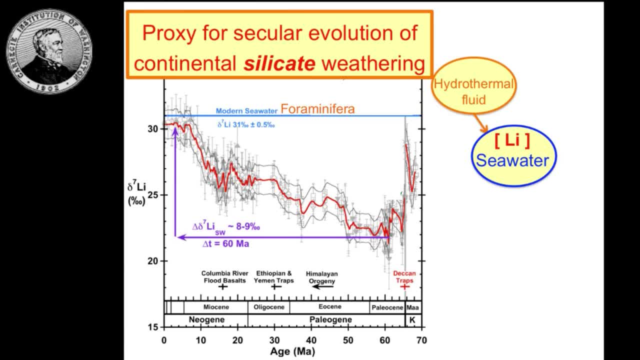 we have lithium and then we have two important inputs, which is hydrothermal fluid as well as the river water, versus also the- You know river water is a common weathering- And also we have output for the seawater: Lithium in the seawater. 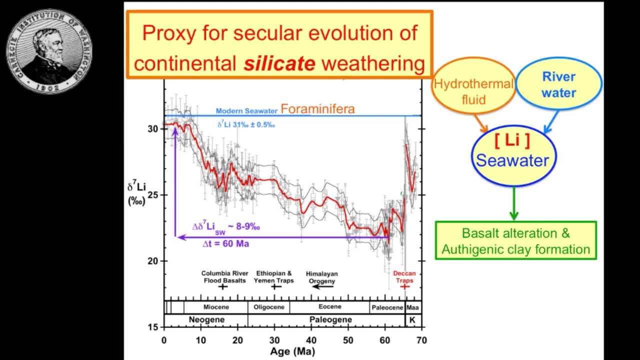 is actually through the orthogenic clay formation and also the salt operation under the seafloor, both of them taking lithium from the seawater. So it's actually not very easy actually to say. However, I would say the hydrothermal fluid is. 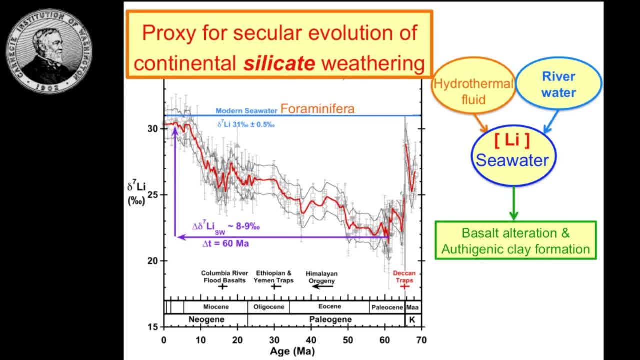 You know, hydrothermal activity is not probably likely to change too much within the 60 million years, And exactly how it changed probably is not well known. And also the formation of orthogenic clays and the salt operation, the mechanism at least not change. 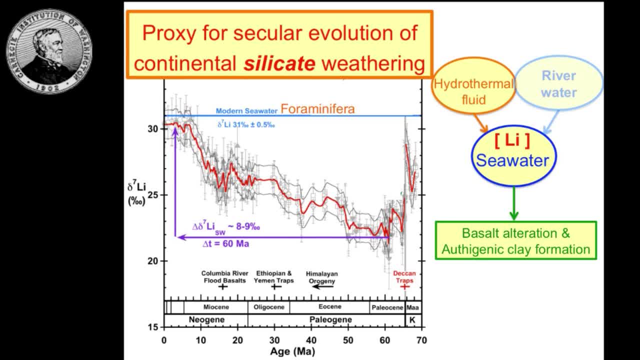 So the most variable part of this is actually river water. As I showed you before, river water shows a large range of lithium isotopic. you know composition. So it's more likely the seawater reflecting the kind of the weathering. the rivering part right. 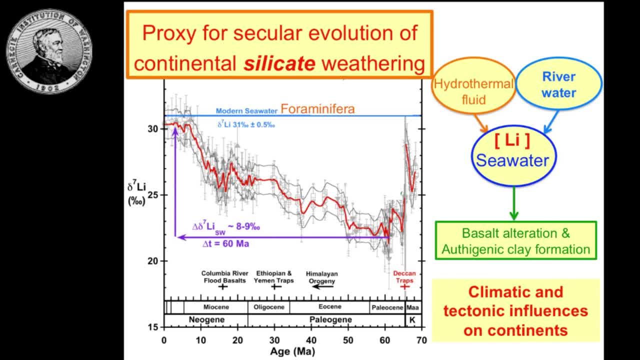 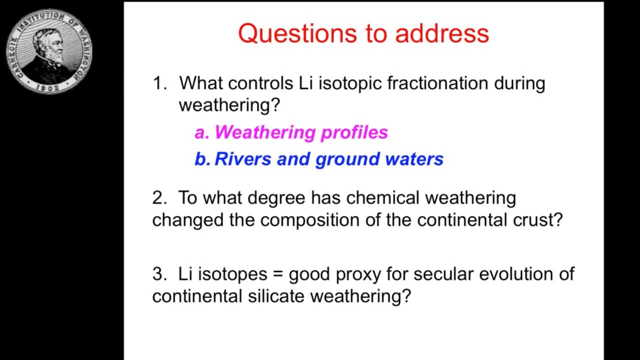 So that's actually helped us to connect between the climate and the tectonic influence, because both of them are important in terms of changing the kind of the weathering patterns. Okay, So this leads us to look at the questions, okay, to address. 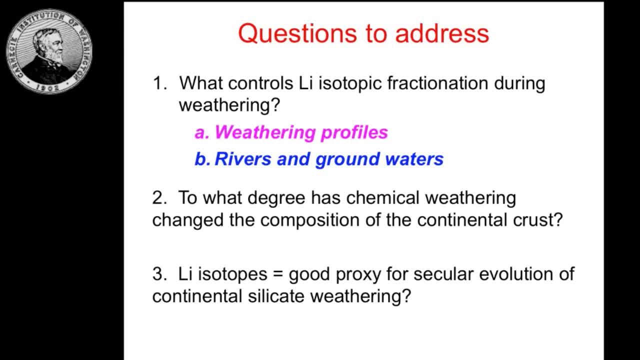 As I emphasized before, we want to know what controls lithium isotopic fractionation during weathering. So there's two kind of study we can do. One is we study the weathering profiles which is left over from the weathering process. One is from the rivers. 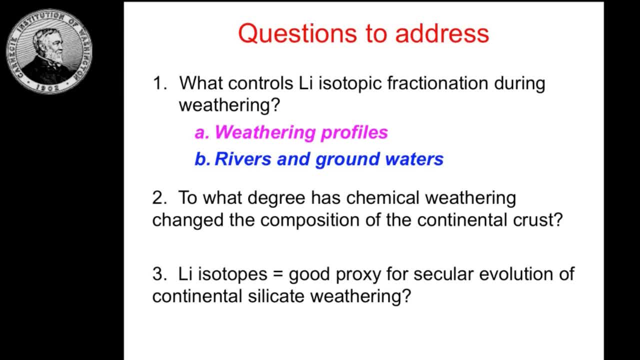 which is taking way into the oceans And also- actually I already emphasized- to what degree chemical weathering has changed. the composition of the continental crust is also important question And also we have potentially good proxies to study the secular evolution of the continental silicate weathering. 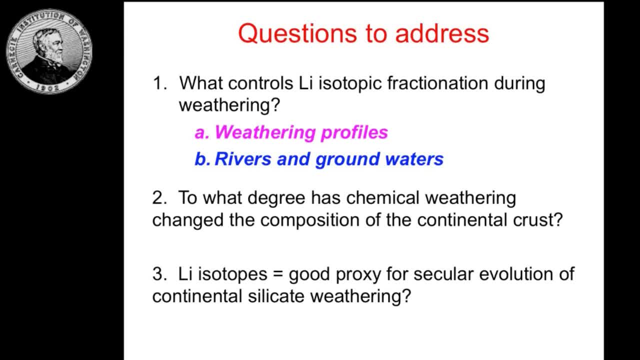 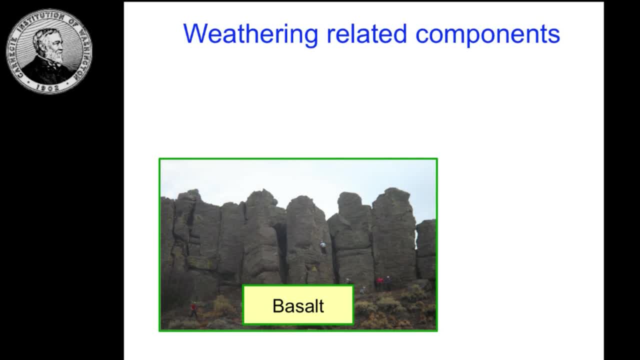 using lithium isotopes. We want to test if this tracer is a good one. So this one. just give you a word of simple idea, right, Since the building block of the continental crust is originally basalt, so we want to study basalt weathering. 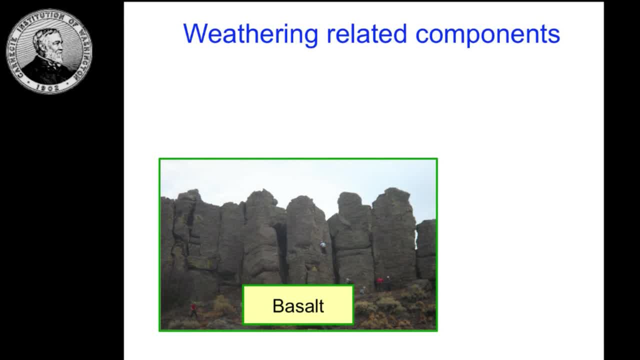 So this is picture taken from the Columbia River basalt. Actually, this is people doing rock climbing in those big columns actually. So actually, if you think anything on the surface of Earth, it's actually been through weathering. So this is a very simple cartoon. 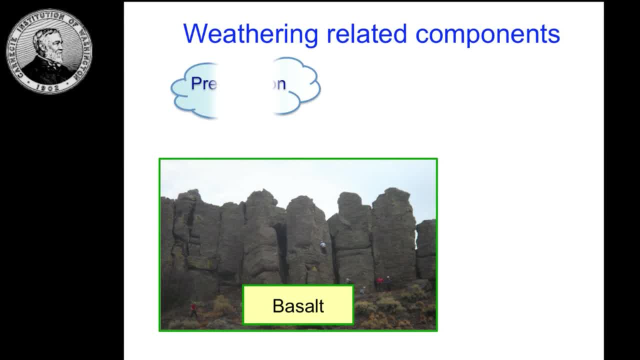 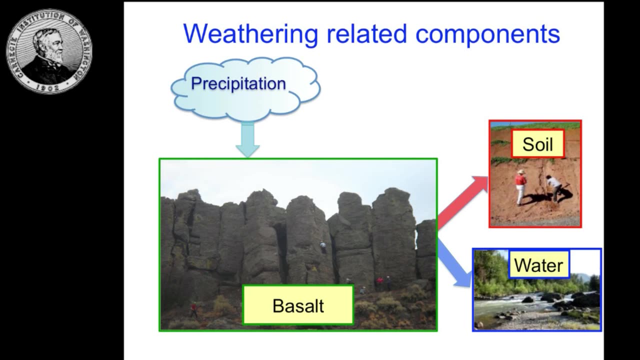 A rock basalt sitting on the surface of Earth right. Then we have precipitation in forms of rain or snow. interact with the rock Fresh rocks on Earth's surface, Then they can produce soils and water. Basically weathered rocks versus water. 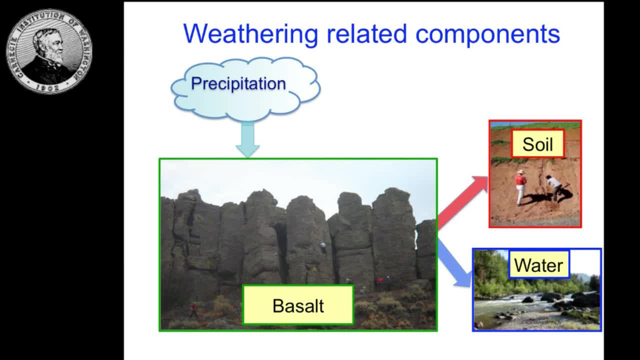 The rocks, the weathered rock or soil or weathering profile, whatever you call it- staying on the surface of Earth and then the waters going away. But yeah, some of the soil can go with suspended as a suspended load into the river as well. 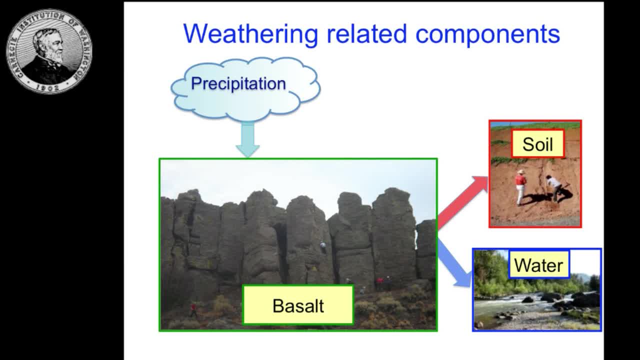 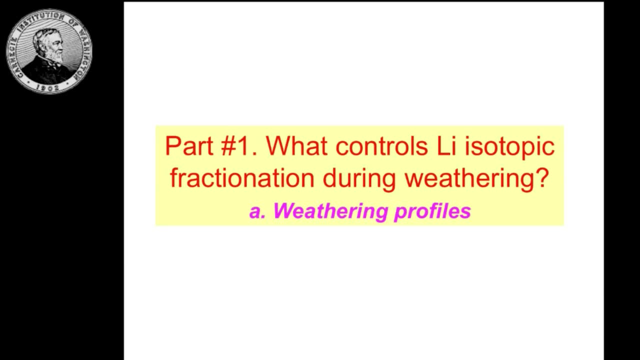 But that's another complication In the meantime. actually, this is not- I want to emphasize, this is not- the open system behavior, because you may have a dust, an aeolian dust component from outside of the system, right, So okay, so we were focusing on the weathering profile part. 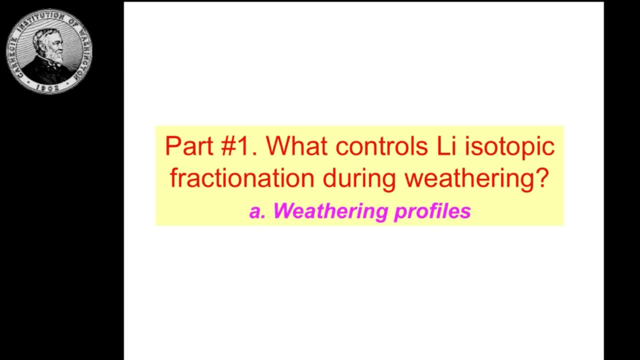 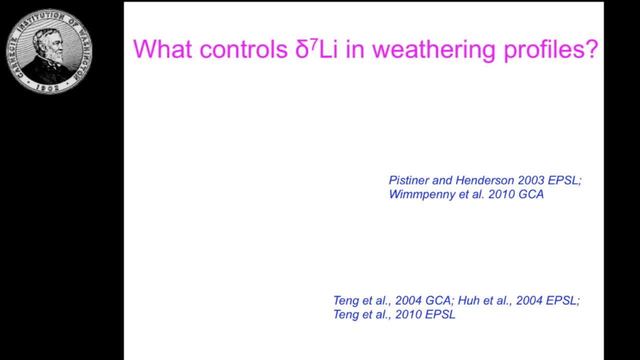 to address the issues of what actually fundamentally controls the lithium isotopic fractionation during weathering. I want to show you some previous study. just summarize: We both have. we both have experimental study and natural observation that no lithium fractionation actually occurs during the primary mineral dissolution. 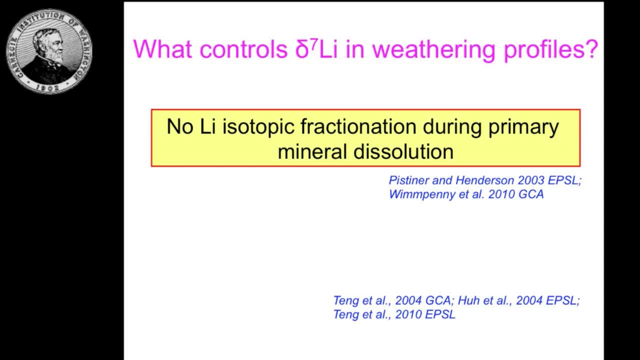 without the secondary mineral formation, right. And then we have fractionation of lithium in the secondary mineral formation. As I showed you, the lower lithium likes to stay in the clays or iron aluminum hydroxide, So they produce low delta lithium signature in the minerals. 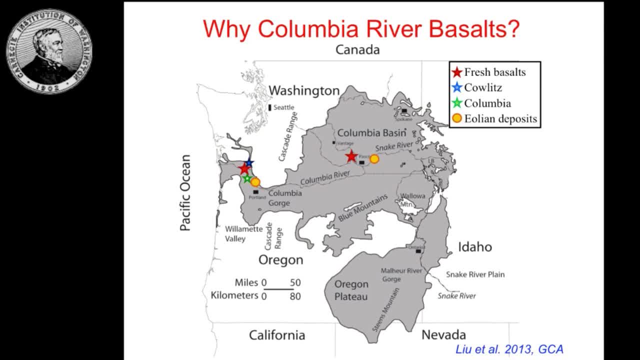 Secondary minerals. okay, So we know that. And then we still want to have a systematic study to look at both rivers: groundwater, as well as the weathering profile, fresh rock from the same system. That's why we go to the Columbia River basalt. 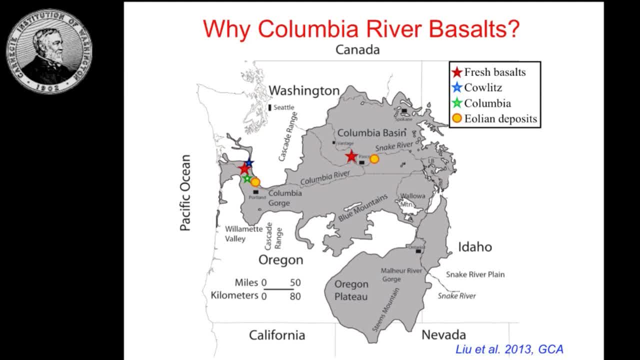 because we need a lot of basalt to look at the weathering. So that's a natural place we can find a lot of basalt. So the Columbia River basalt system is located in the Washington state and also Oregon and a part of the Idaho. 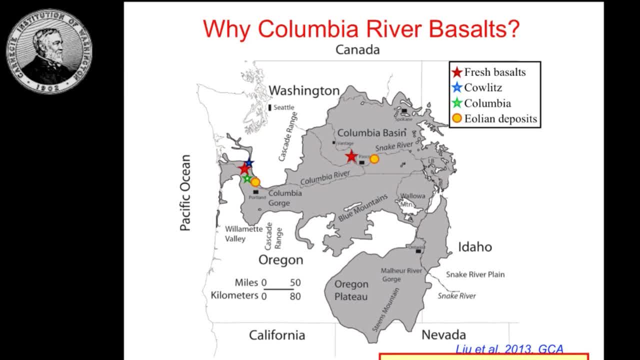 as you can see, it's a large igneous province And it was erupted in about 60 million years ago, because the basalt showing in this gray here are widespread and also well studied, So we can look at the weathering, because we know their parents pretty well. 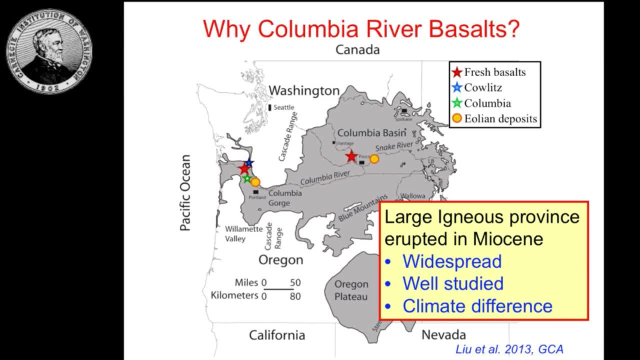 And also we have a bonus in terms of looking at the weathering system here, because the rise of the cascade having the mountain shadow effect making the climates to be different in the west and in the east. So we have more precipitation, more than about 2,000 millimeter per year, in the west. 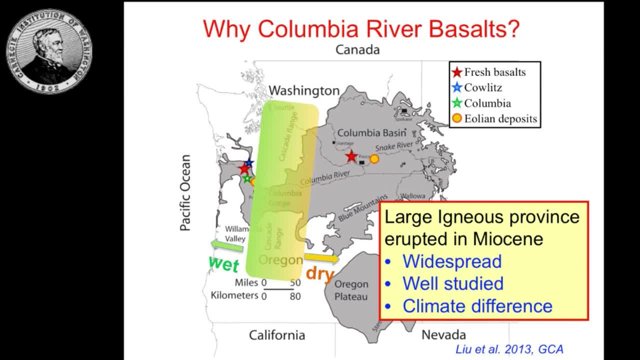 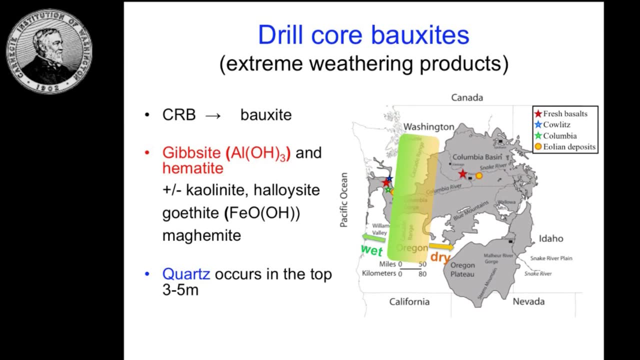 And then we have pretty dry- less than 300 millimeter per year in the eastern part of the Columbia River, So we can look at the weathering from different climatic conditions. Okay, so we, as I promised we will study some weathered rocks, right? 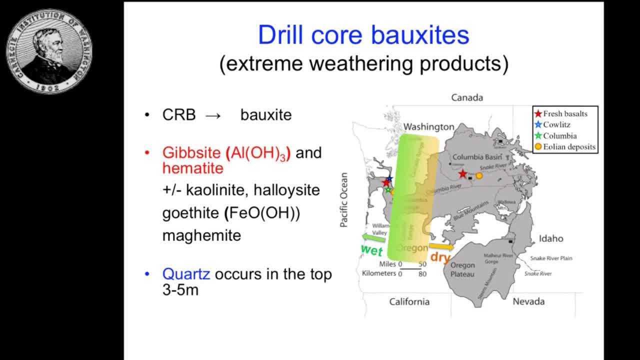 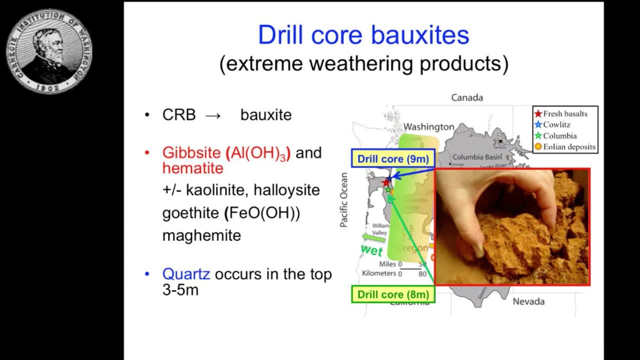 So we got some drill cores. They are already box size. So what is a box size? They are actually extremely weathering product. Looks like this: Very, very aluminum oxide and also hydroxide rich. Basically METO XRD shows. 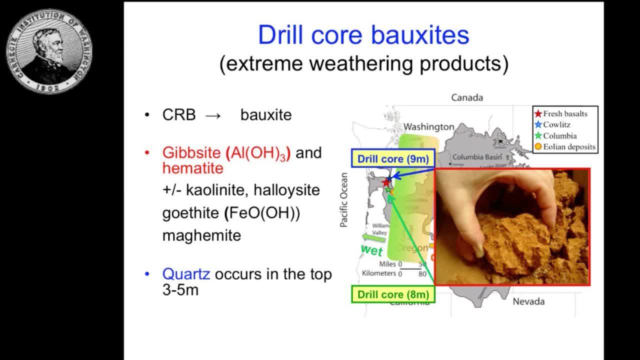 majority of them are METO deep side and hematite And we sum a little bit kaolinite or other clays and iron hydroxides. So those two drill cores are from the west of the cascade, So they are from the wet weathering right. 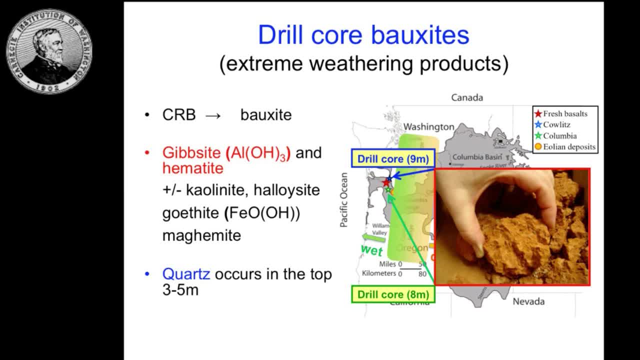 And they are from the drill cores, about 10 meters in length. What's interesting is we found the cores on top of the three to five meters of both the weathering profiles. So cores, as you know, is not supposed to be the primary mineral. 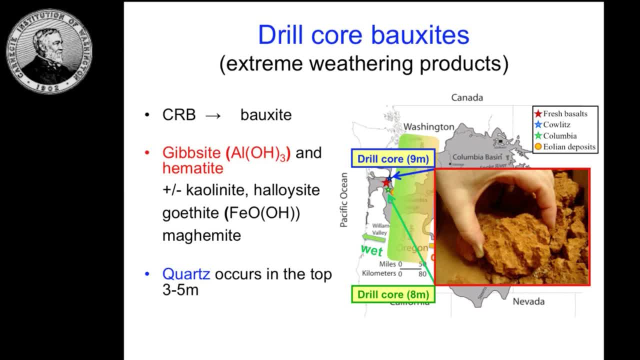 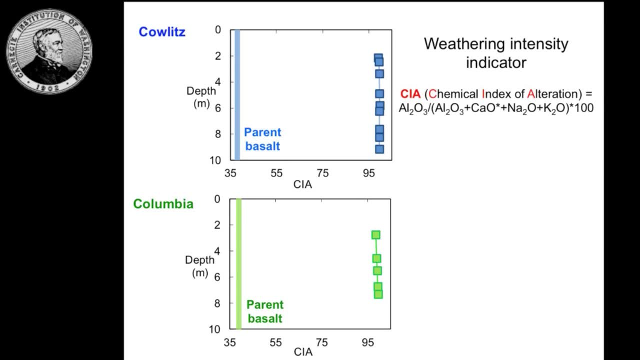 for the salt right. So that's our first hint if something is going on And also if people study weathering processes. we like to use this term CIA, not the agency, but the chemical index of alteration. So this is basically aluminum content. 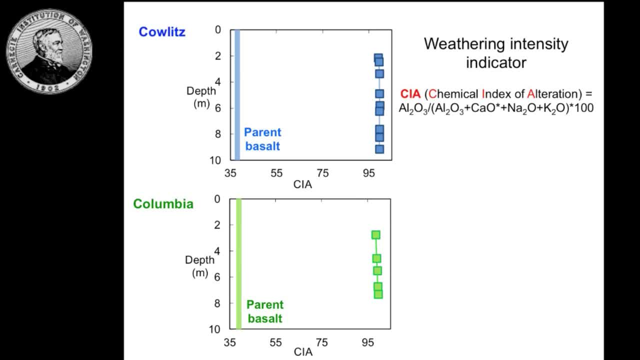 versus some alkali element to indicate how much of the rock has been altered due to fluid or interaction right. The more aluminum you have, the more weathering has occurred because you lost all those mobile elements, soluble elements, As you can see, I mean. 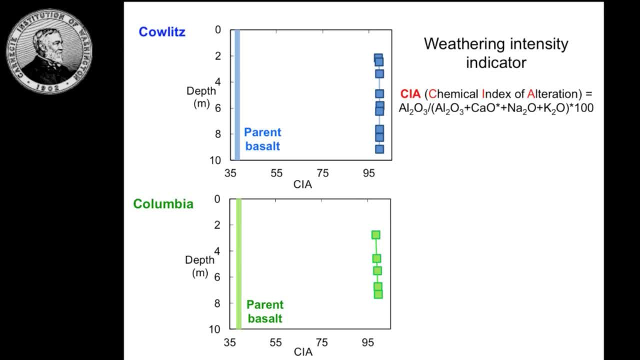 all those boxes are the box size, the weathered, very crappy material, And then those bars indicate the parent material, which is the basalt, And for both the two profiles, both kaolites and the one called kalimba. so that's about two different weathering profiles. 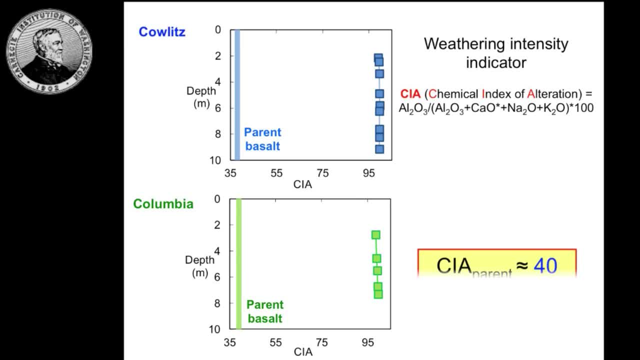 I showed you before. So all of them showed a very homogeneous parent: 40, and then the box size showing 99. So 100,, as you can see from this equation, is the highest you can get right. So 99 is, as we say is, extreme weathering. 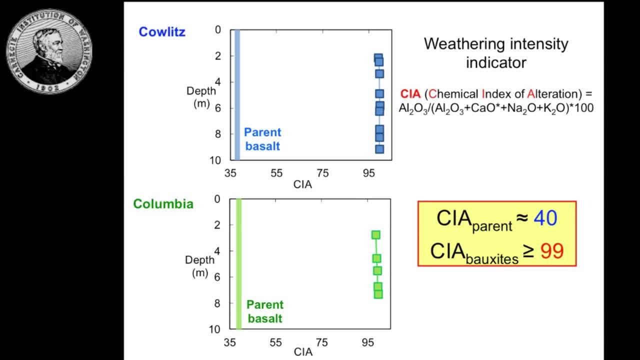 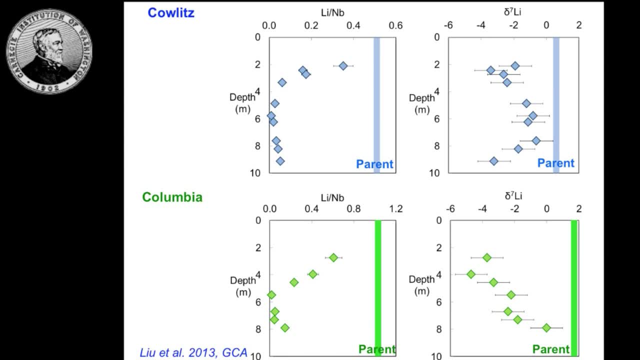 But, as I want to point out, we cannot distinguish all those samples in the box size because they all look the same- all extreme weathering. So we did this lithium study to look at how they behave during this extreme weathering. right, And it's the same profile. 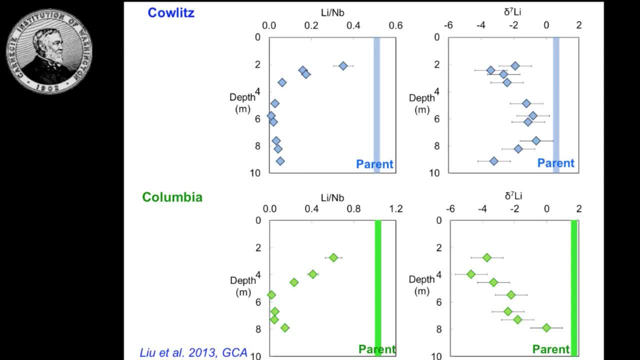 for both kaolites and the kalimba, where we have the parents in the bars characterizing the uncertainties in the bar, And also we do the delta lithium. As I showed you, the definition is the same as other stable isotopes. 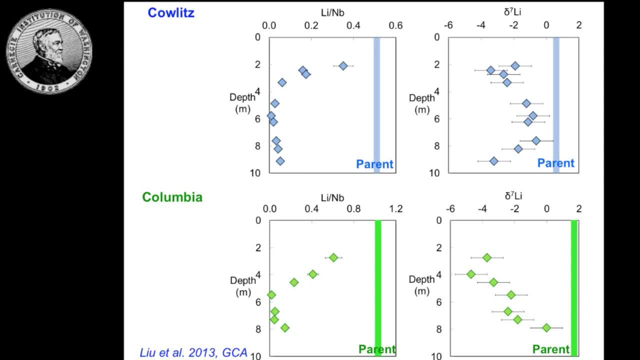 So first of all we see there is a depletion of lithium content in the box size compared to the parents, And then we have a systematic kind of decrease for the isotopic composition, right? So this we can try to explain, right? So the first depletion we can easily explain. 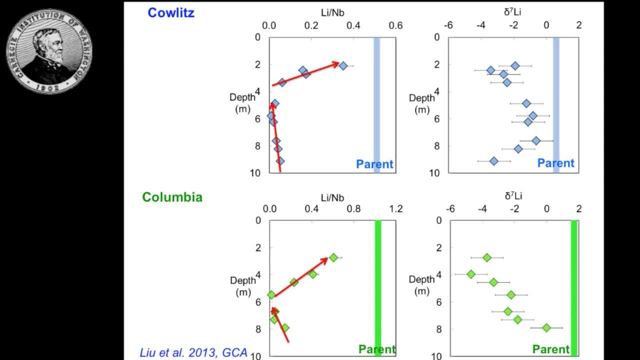 because lithium is a soluble element, right? So it's of course lost during weathering. However, the top enrichment is not known. So for the isotopic value, as I showed you before, the fundamental fractionation of lithium isotope: 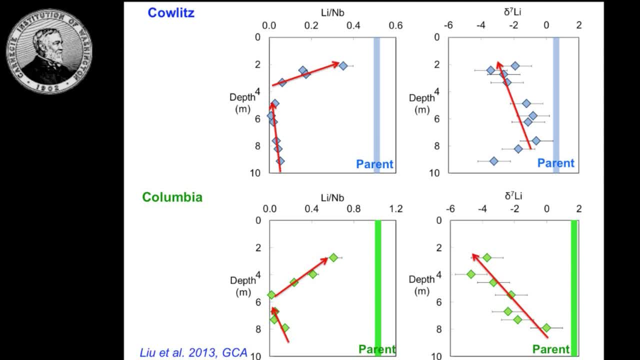 is the secondary minerals or, like clays or iron oxide, prefers the light lithium. So it's not surprising we have a sort of upper rising, you know, decreasing delta lithium with depth because it gets more weathered on the surface. So but then the enrichment here is not explained. 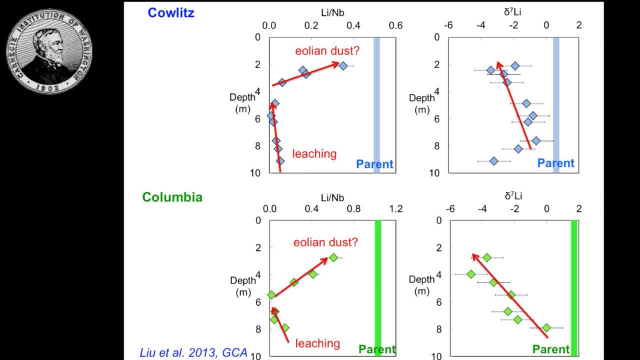 It could be due to aeolian dust component, And this one is due to secondary mineral formation. So we can explain this all but the aeolian dust. we cannot be for sure because you know, lithium could be behaving not homogeneously. 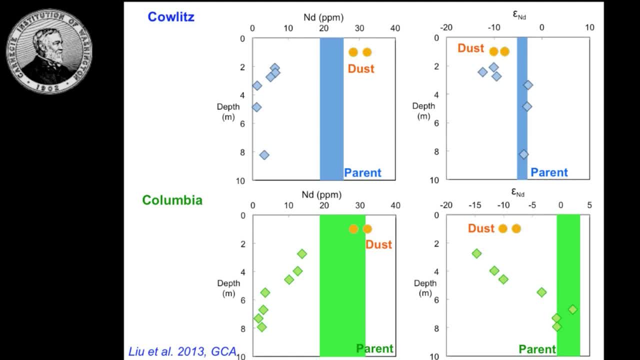 So we want to do a more definitive study focusing on neodymium isotope, Because neodymium isotope is a good tracer to study the source, So we can analyze all the parent material and also the box size in those diamonds And also we analyze the dust sample we collected. 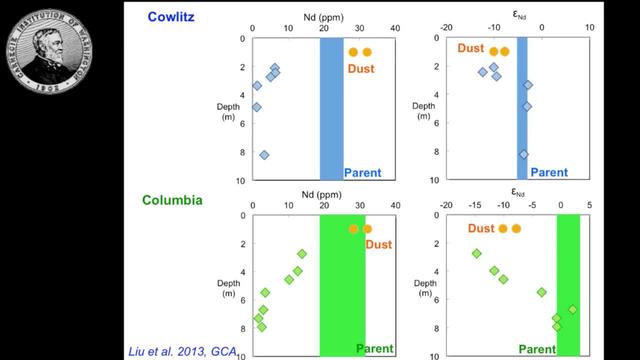 from both west and east sides of the Columbia River, We can see clearly. first of all, it's very surprising because sometimes people claim that neodymium is not mobile during weathering, But in this extreme weathering case the neodymium is actually depleted in those box size. 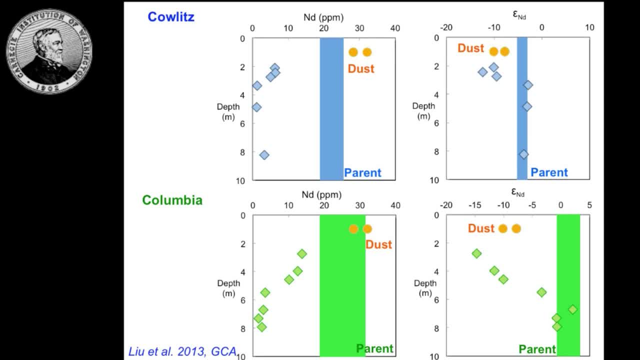 So the parents are showing in those bars right? The second important point is we have seen the dust having less radiogenic signature, as well as those top three samples from both profiles showing similar less radiogenic signature as the dust, And also the bottom profile showing similar signature. 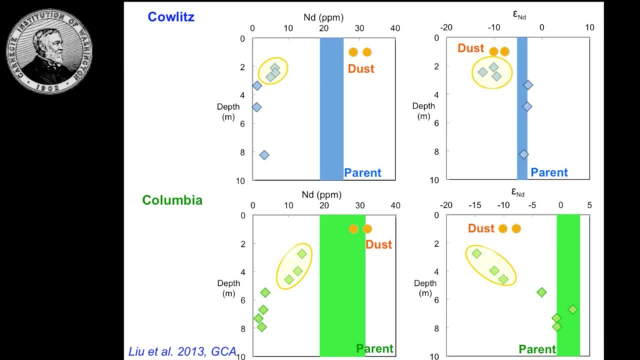 compared to the parent right. So that's actually very good, because those samples corresponds to the ones that we did the XRD. So those are having cores in their mineralogy. So that's a more definitive proof that those are likely from the aeolian dust component. 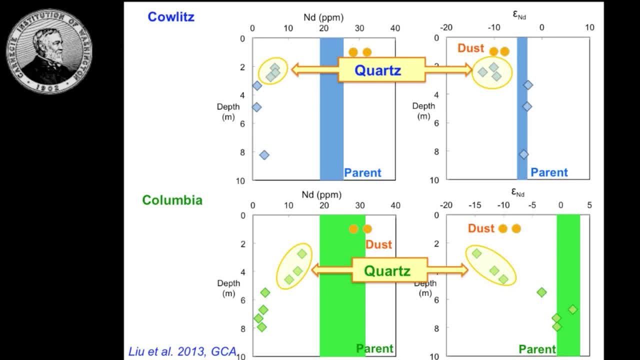 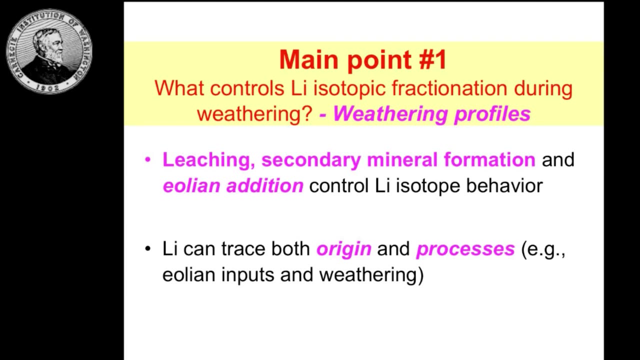 for those top samples where we see the lithium enrichment as well. So just to want to mention this is important When we talk about the lithium isotopic fractionation in the weathering profile. Okay, so just the main point I would like to show you. hopefully you're convinced. 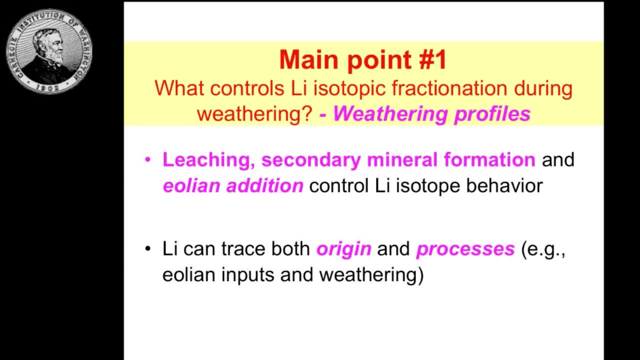 both leaching secondary mineral formation as well as the aeolian dust. addition controls the lithium isotopic behavior because weathering is an open and a dynamic system, So lithium can have a capability of trace both the origin and the evolution processes. So that's good. 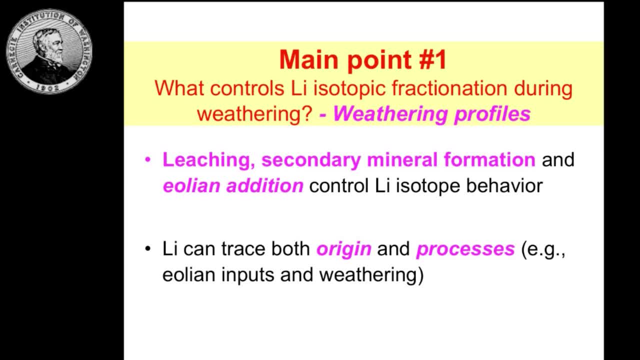 Is the grain size of the quartz consistent with it being dust deposited? Yeah well, it's actually harder to see. We didn't see it, It's all. the material is all crappy, So we didn't do the thin section analysis. 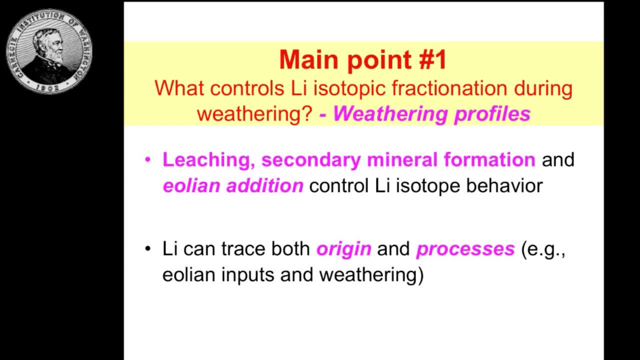 So we just we had to crush the whole samples to powders, go to the powder XRD, So it's hard to know the grain size. so, yeah, Okay, Did you measure the lithium isotopic composition of the dust? Yes, we did. 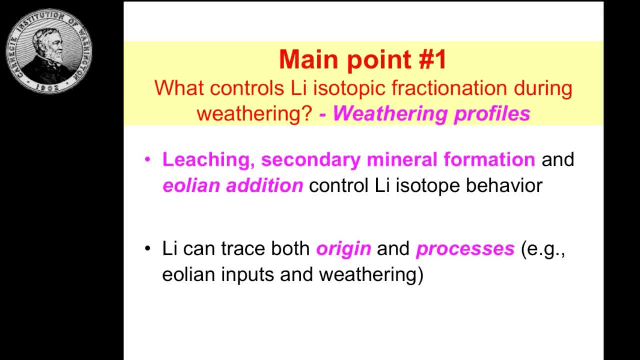 What was it consistent with? Did you show that here? Oh yeah, I probably did it. Well, yeah, it's also. it's lower, So it's close to the upper, kind of crust, So it's around. one of them is negative one. 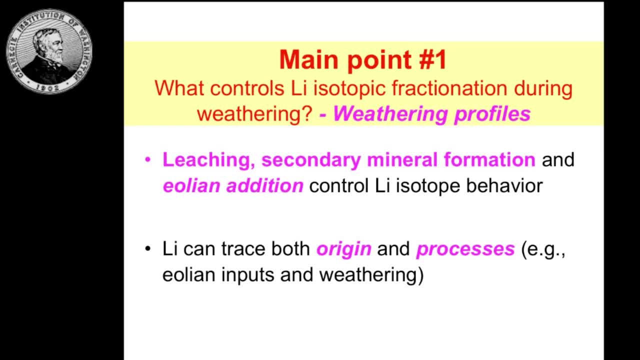 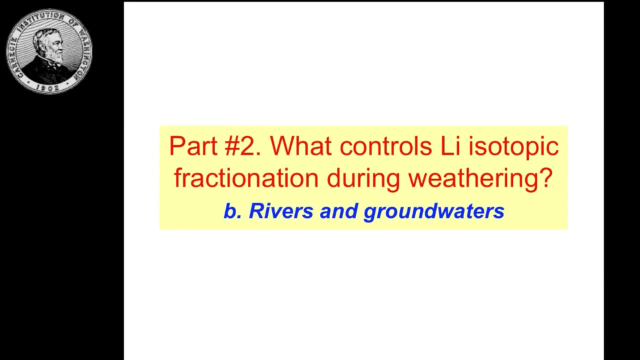 one of them is positive one, So it's zero plus minus two within the upper crust range. Good point, I didn't put it out, So you're ready to get a little bit wet after this? So and then the second part. 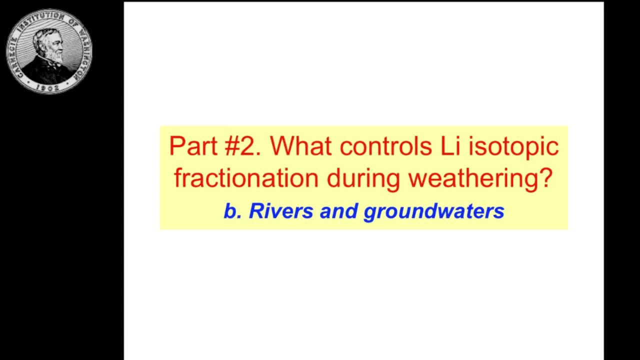 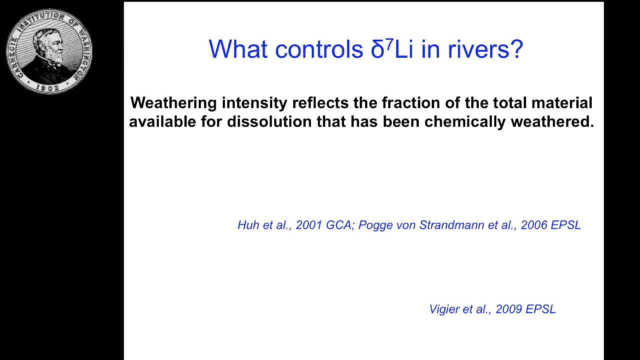 I would like to address the what controls lithium isotopic fractionation. looking at the rivers and ground waters, So that's the wet part, Okay, So we know what controls lithium, sort of. Before that, we want to give you an introduction. 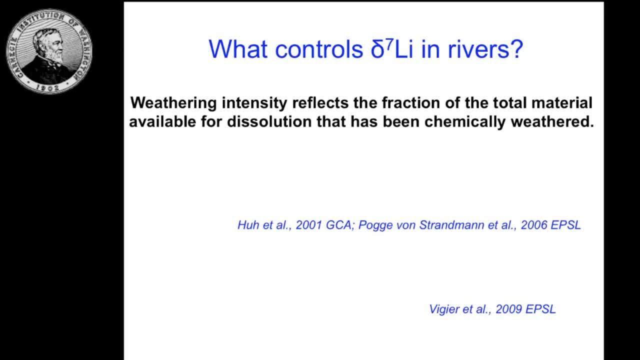 of this definition of weathering intensity. So people talk about this all the time. It's basically reflect the fraction of the total material available for dilution that has already been previously chemically altered, right? So the higher the weathering intensity, meaning the sample already been through weathering. 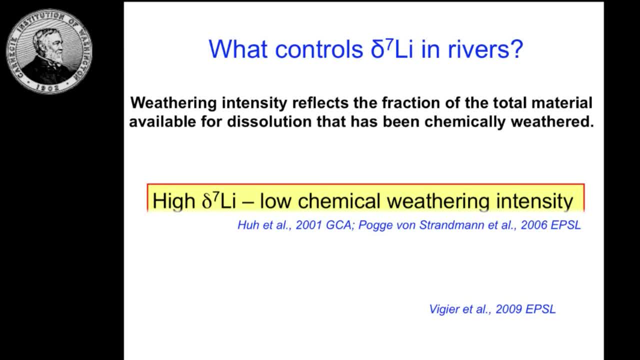 However, we have two different schools of what controls lithium in rivers in the literature, because some claims that the high delta lithium is usually correlated to low chemical weathering intensity to rain. where they found there is high delta lithium values in some Andes rivers that are draining Andes in the Amazon. 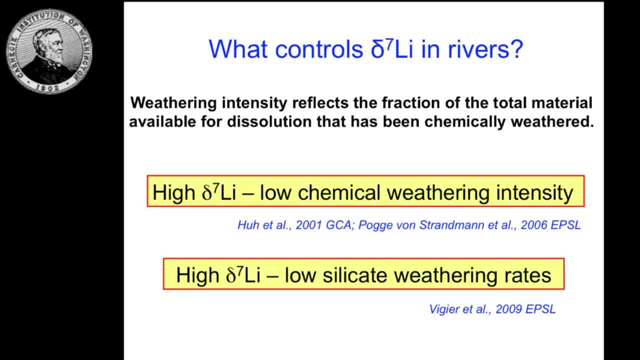 And also some claim that high delta lithium may reflect the low silicate weathering rate. right, This intensity is accumulated effect, but rate has the time component. It's basically correlates with the flux. So we want to, we want to look at the lithium isotopic behavior. 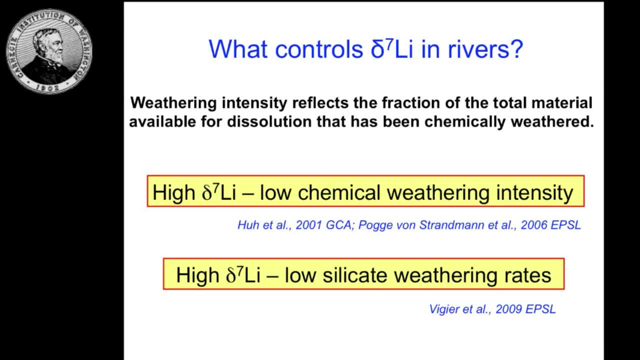 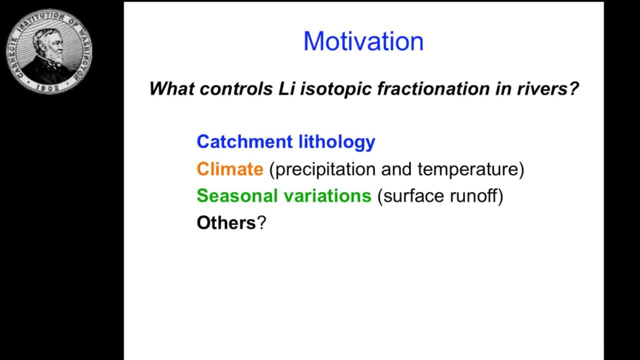 to see what actually controls the lithium behavior by a small rivers. So this is our advantage of doing this kind of study because, as you know, we're focusing on the Columbia River salt system. We already characterized the weathering profiles, as well as the parents. 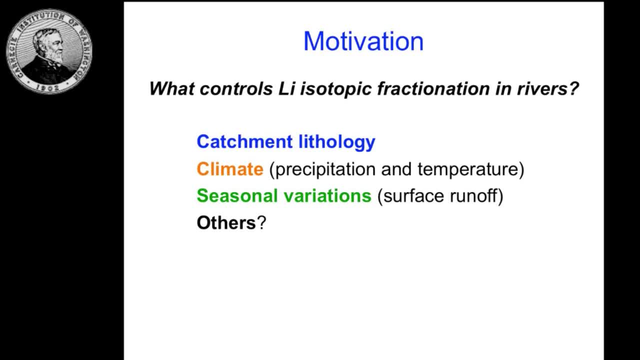 the potential dust component And also we can keep the catchment list solidly- the same right. So the catchment list solidly is important factor in influencing the what's dissolved in the river. So if we keep everything is basalt so we get rid of other factors influencing lithium behavior. 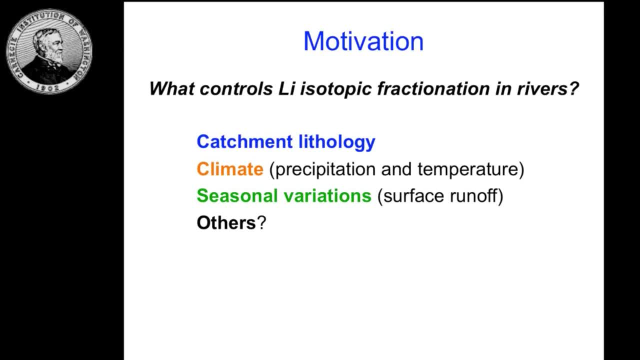 And also climate may be important, because there is different precipitation and temperature may have different lithium isotopic behavior, And also we would like to address seasonal variations. right, If you take a, you never you know. there's a saying: you never walk in the same river twice right? 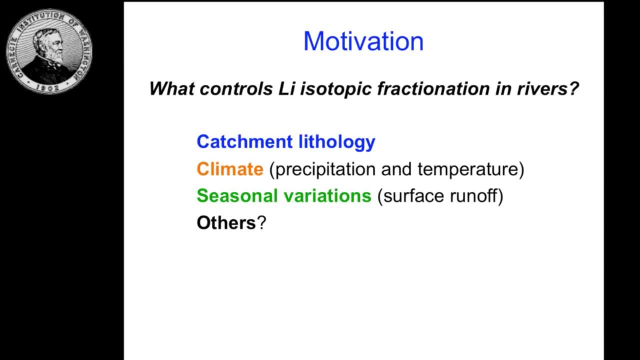 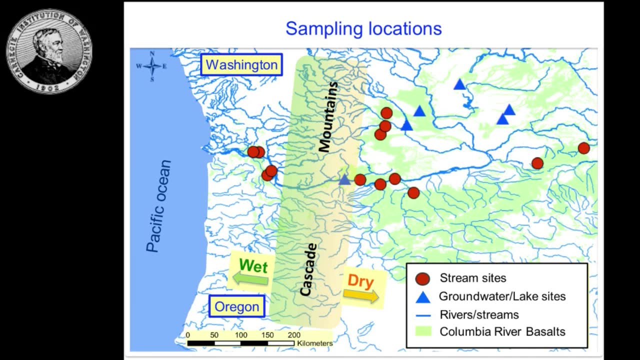 So there's always seasonal variations possibility. So this kind of motivate us to try to invest rivers and the ground waters in the single lithology catchment, which is the Columbia River salt, where you can see it here. So we did a geological map of the salt exposure. 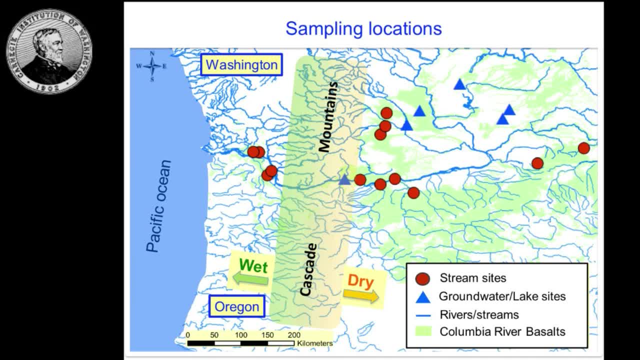 which is the light green in this area, And then on top of a hydraulic map. So those are the positions. we took samples. So all the orange circles are the rivers, or maybe we should call them streams. As you will see, those are only meters cross. 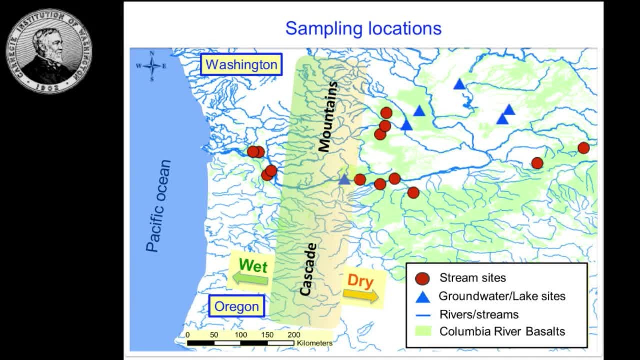 Those are not real big rivers, Those are small rivers. The point is they are all weather the light basalt, So we don't want to have other components. And also the triangles are some ground waters we took in the basaltic terrain. 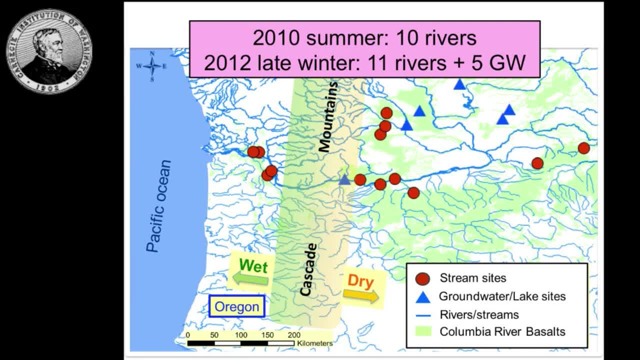 So we also do this in two different campaigns. We do it in summer- very nice and kind of cold- late winter as well- to sample the same streams and ground waters. I just want to give you an idea, since we are not there. 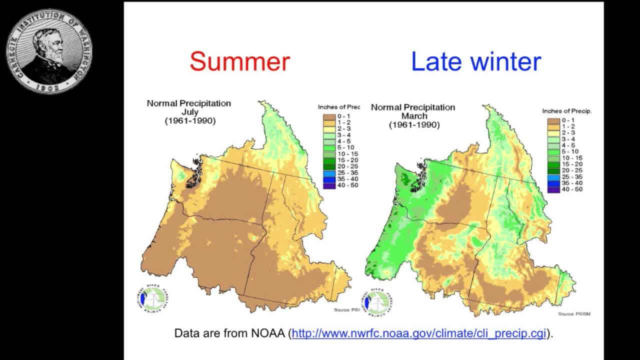 give you an idea of the Pacific Northwest of the climate. right, It's actually very interesting, For the summer it's all dry And the late winter, the west part of the Cascades- it's actually very wet, So the precipitation was higher. 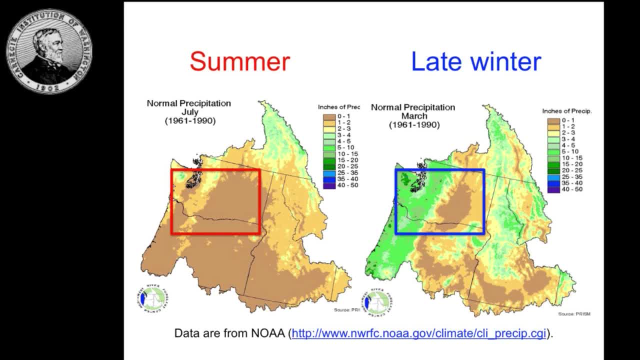 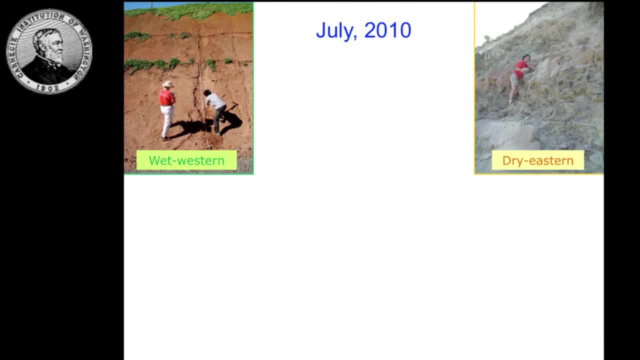 So remember that. So that's our study area, That's the Columbia River basalt area. So just keep that in mind. So there's some fun- always fun to have some field photos. That's a very nice summer photo In the west. 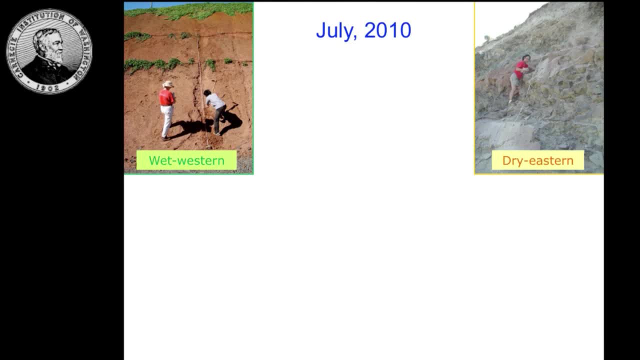 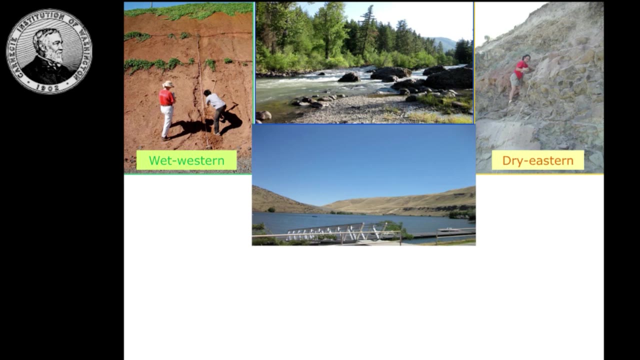 you will see some soil development, red soil- And then in the west there's hundreds and hundreds of meters of basalt. So a lot of basalt In the dry eastern area. So we took some river samples as well in relatively west. 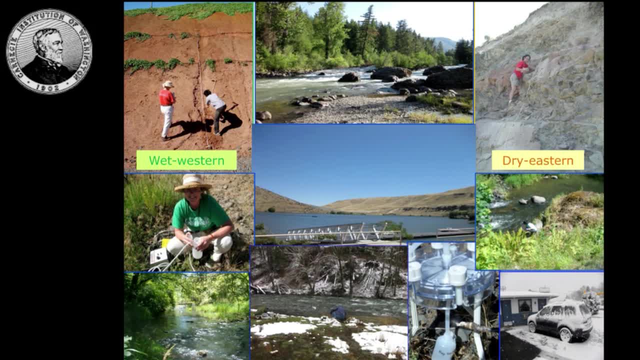 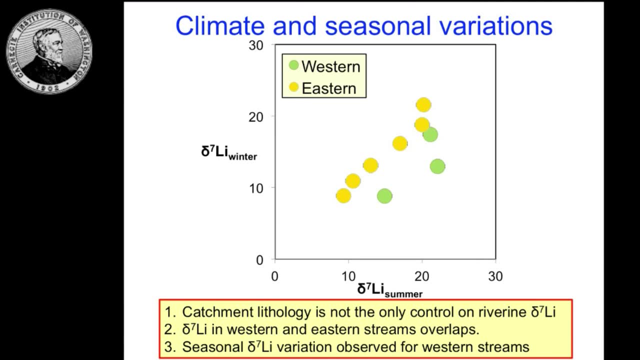 and also the east samples, And also in the cold winter where we have snow. Okay, now we look at the data, Because we did the two different seasons- One is called winter, one is summer. So we plotted winter Duluthia versus summer. 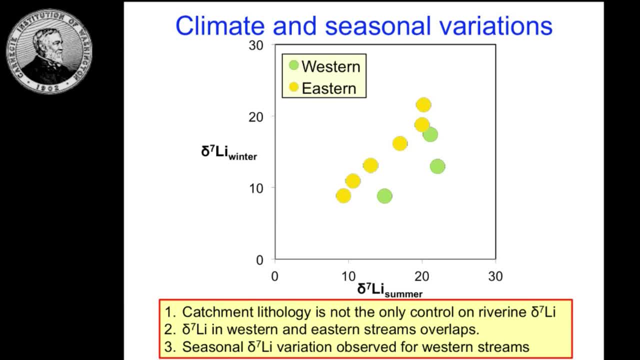 And also because the locality we have the western and eastern river, So the western river are shown in the green and eastern are the yellow, The first thing you can see, no matter in summer or winter. there is a large range for the Duluthia value. 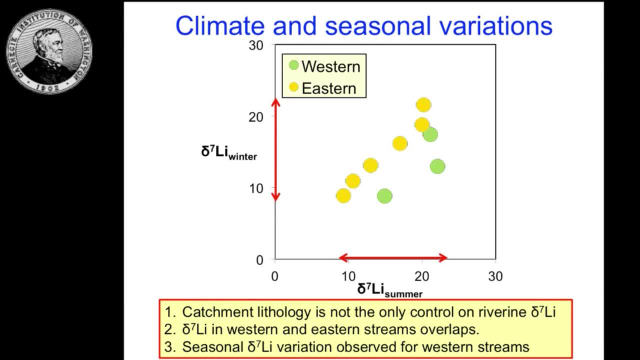 Even in those very small streams that we think is only weather basalt. So that's surprising. And the other thing is, if you look at this long time enough, like me, probably- you can see there is a one-to-one line. 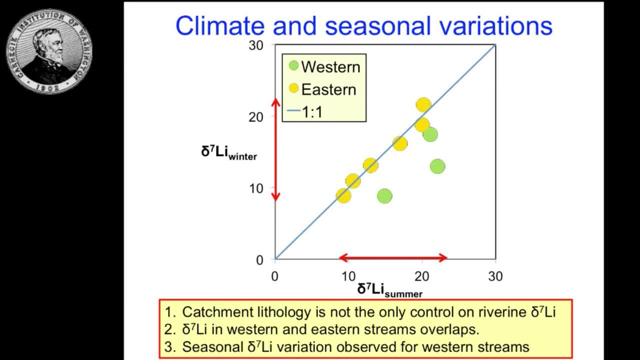 on those eastern rivers. What falls on this line means there is a same. there's no variation between the summer and the winter, Duluthia right And all the western rivers showing the heavier values in the summer. So that's another interesting observation. 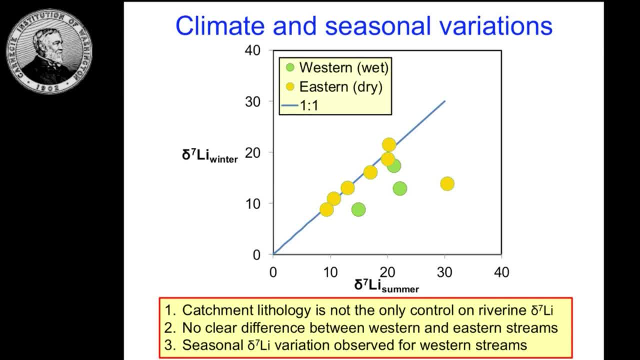 But if you do the math, if you do the math correctly, I had done 10 rivers twice. So I only showed, like here, only nine points, right? So there is only one off. So that's the honest point, right? 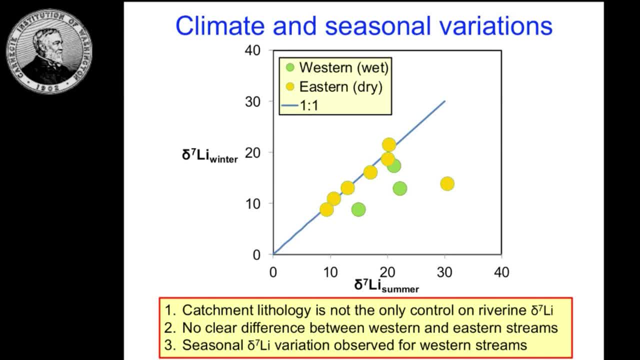 So in the suffering season actually we saw cow poos in the stream And also because we did all the major cation and anion analysis, we found there is a huge amount of chlorine and sulfite in those waters, So there is possibly fertilizer contamination. 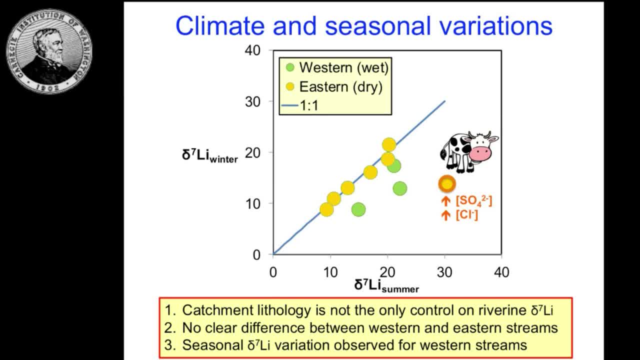 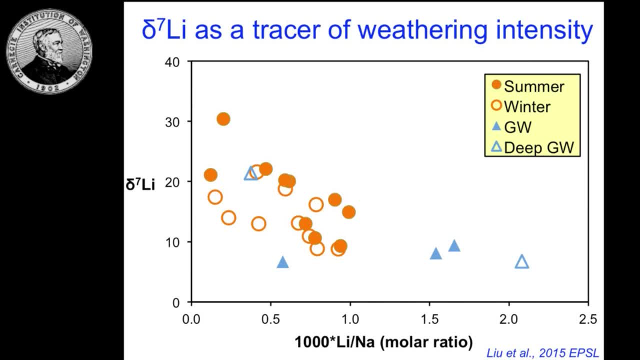 or I don't know, cow pojetic contamination, So we don't want to talk about that too much. Okay anyway. so if you look at the whole behavior for both summer and winter, for the streams shown in those circles and also the groundwaters showing in those triangles, 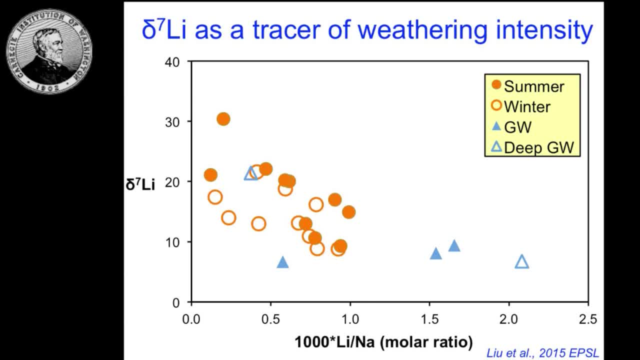 I would like to mention there are some deep groundwaters, actually meaning a couple hundred meters depth into the salt, So actually their residence time is probably thousands of years, So they are actually not reflecting what's going on now, So that's why you probably have to look at it in this way. 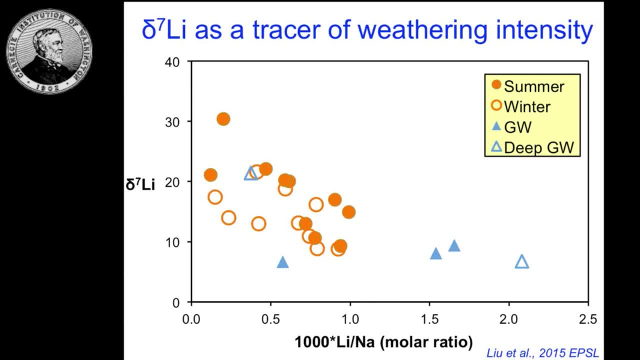 But anyway, if you look at this behavior of lithium concentration versus delta lithium- oh, by the way, we would like to normalize it to sodium- It's because both lithium and sodium are soluble elements But have similar solubility, Lithium for first, goes into the clays. 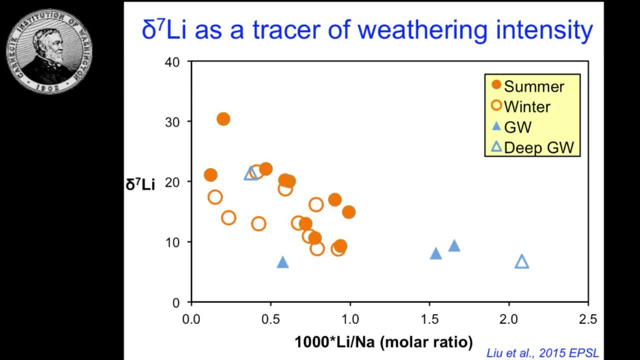 Sodium, not much. So this is an indicator of how much of additional weathering going on in the rivers that we like to use. Anyway, if you ignore, there's kind of statistically four samples, but it's very hard to get groundwater data right. 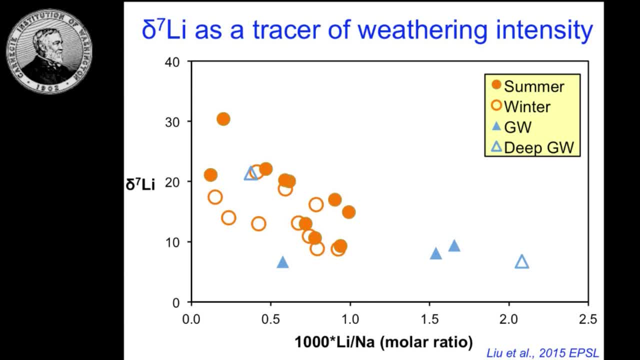 Some of them, we actually went to a bathroom faucet. We know that there is a deep groundwater wall, But anyway. so despite this, there is one deep groundwater that doesn't follow, Majority of the streams actually having heavier values compared to the groundwater right. 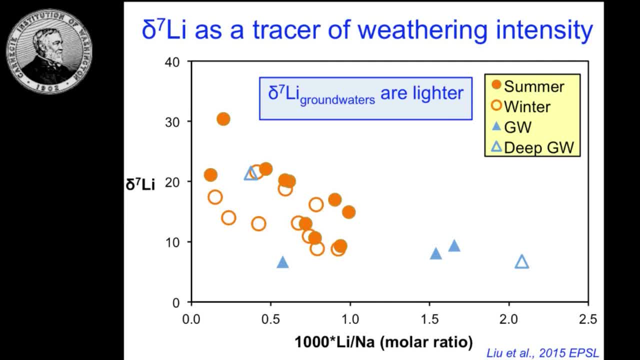 So that's our first observation, And also there is seem to be a trend of this increasing delta lithium with lower lithium-sodium ratio, where previous people are thinking there was maybe a mixing or two different weathering regime, meaning one of them is probably formed. 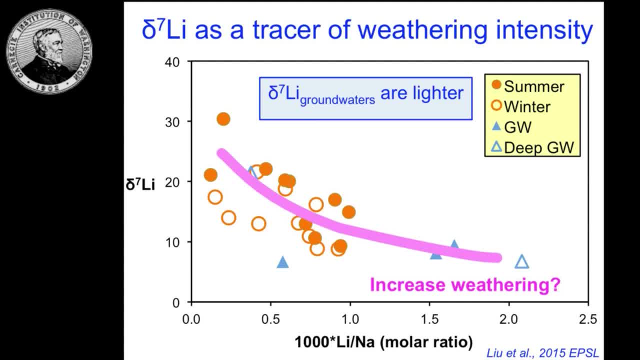 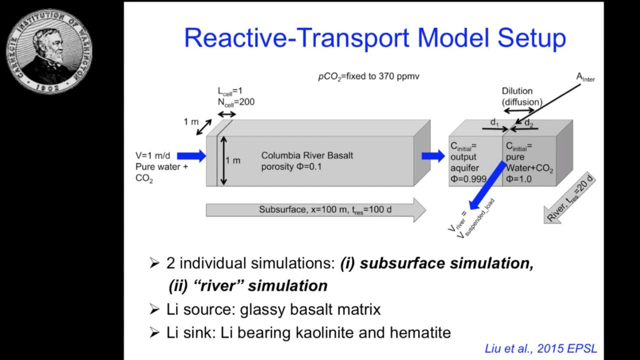 by secondary minerals and the other one is probably by manganese oxide or something. But we were trying to explore this by some models. So this I'd like to give my collaborator, Chris Warner, a credit. He did basically this reactive transfer model. 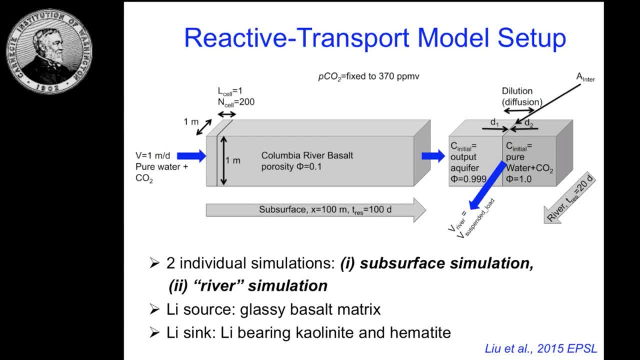 by looking at how the pure water plus some CO2 going through a Columbia River basalt rock. We gave it some peroxy, So the water going through with some residence time and then coming out. So this part is actually simulating what's going on in the groundwater. 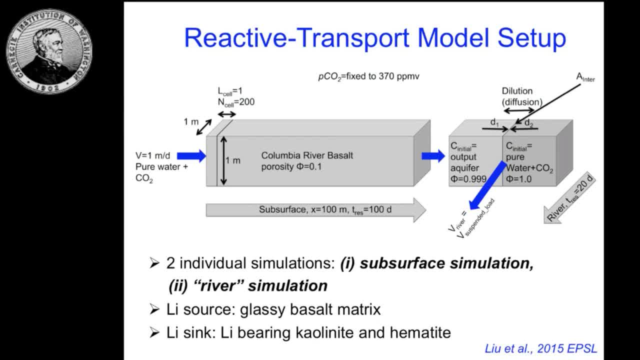 right subsurface, And then this groundwater comes up and then mixed with some freshwater. This part is simulating what's going on in the precipitation right by the rain or snow, And then this is what's going on in the rivers. 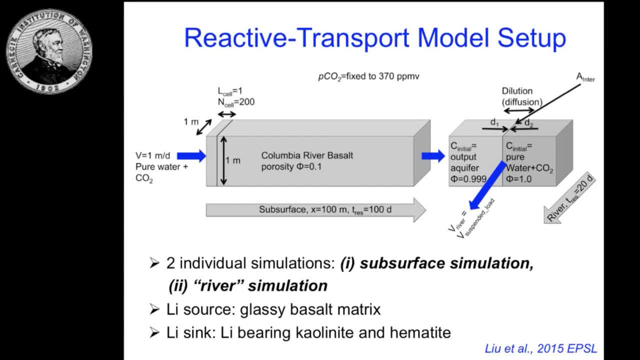 We tried to simulate that. So we did these two individual simulations, both for the subsurface groundwater and also the river simulation. For the source of lithium we used the glassy basalt because lithium is a relatively incompatible element, so it goes to the glass. 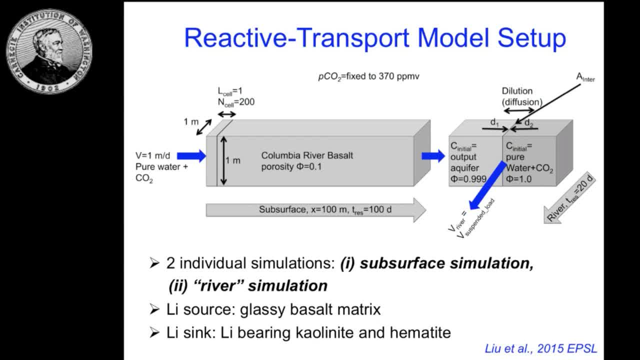 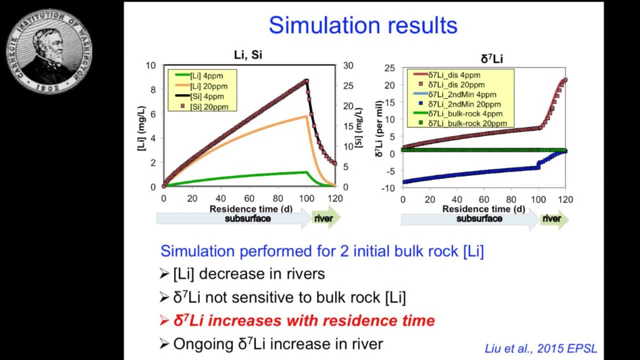 for those high-temperature geochemists. And lithium is sparing, actually in the secondary minerals. We assume it's in the kaolinite or hematite. Then we kind of look at the simulation result for two end members where we assume a low lithium concentration for ppm. 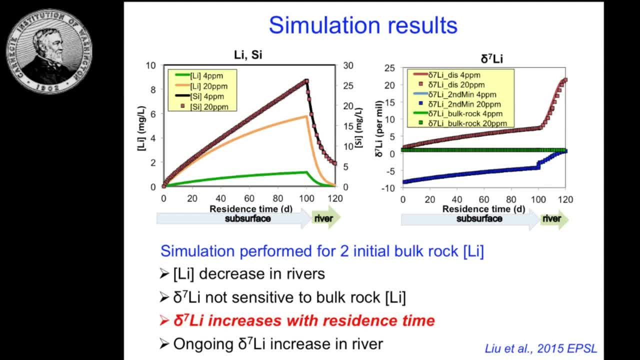 and then a high lithium concentration is 20 ppm for the basalt, because we actually measured the basalt so we know that's the range we observed. So, if you can see, this part is for the subsurface, which is the groundwater. 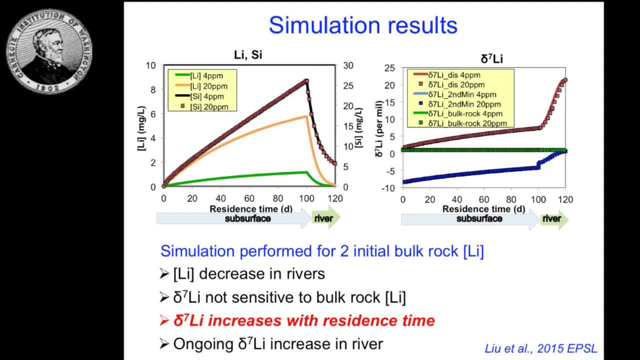 and this is the river right, So in the groundwater, with longer residence time, it's not surprising. we release more lithium and also silicon into the rivers right, So, that's Sorry, into the groundwater, so that's not surprising. 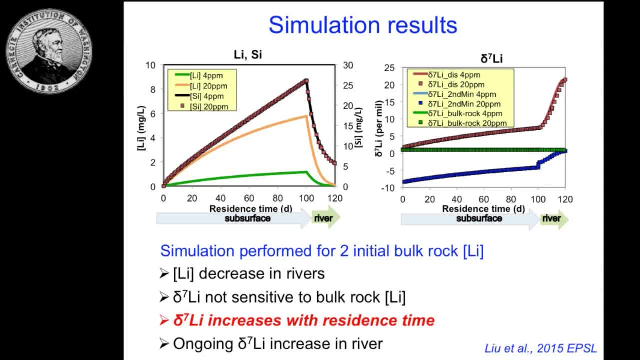 However, because there was a mixing of fresh waters in the river. so we see the decreasing behavior for both lithium and silicon content in those simulations. But if you look at the delta-lithium part it's actually not too much different between the two different starting compositions. 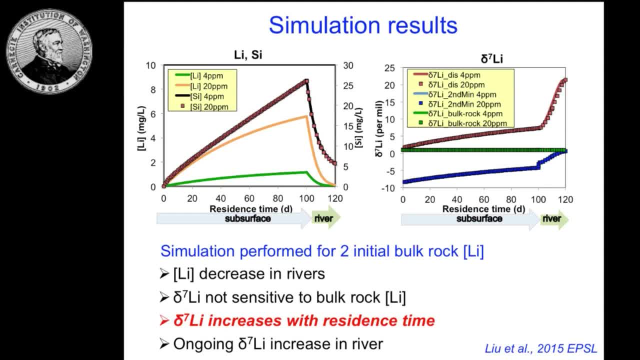 So no matter if it's lithium, which is 4 ppm lithium, or 20 ppm lithium in the basalt, all those behaviors are the same right? So all the rivers show a slight increase in the subsurface and then a huge increase in the rivers right. 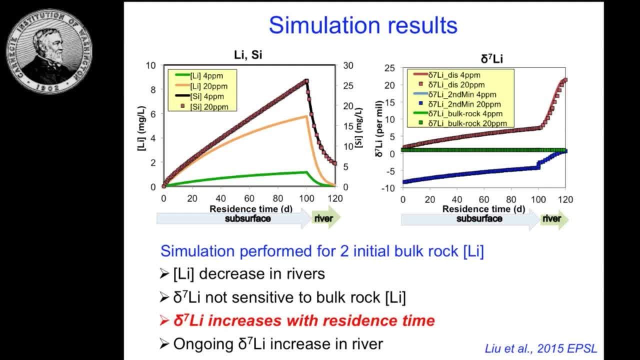 So, if you remember, like my previous diagram, it's an opposite correlation between the delta-lithium and the lithium concentration. Actually, that's exactly what we observed And we would like to point out that there is a very delta-lithium increase. 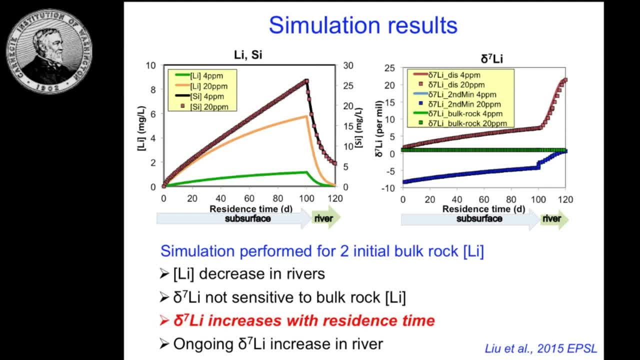 with increasing residence time. So we would like to argue it's actually the residence time. the hydraulic process controls the lithium isotopic fractionation in the rivers, so you can have the huge range. And also the other important funding for this simulation is we see. 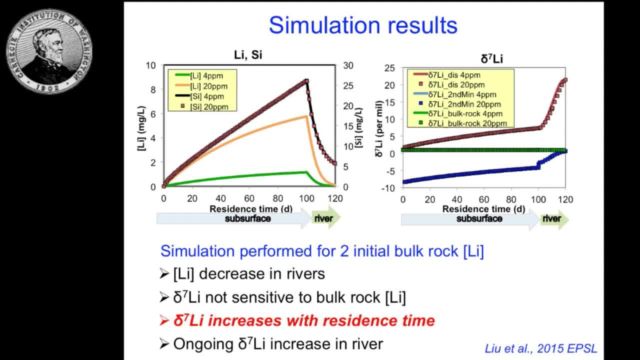 there is additional weathering going on in the rivers right, So that's why we can explain why our river samples have higher delta-lithium compared to the groundwaters. So all the rivers do have higher values. No questions, Fair as mud. 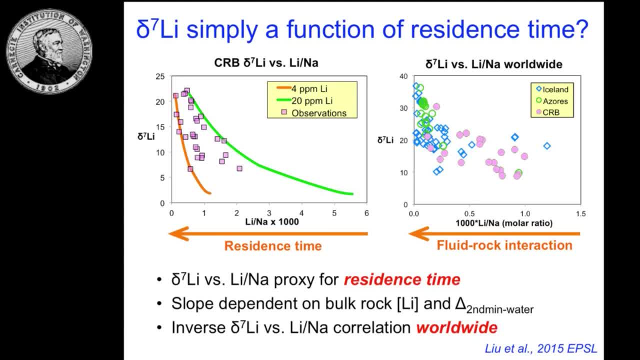 Okay, So if you're not so convinced, we tried to really process to what we observed. So all those pink squares are the observations for both seasons, as well as rivers and groundwaters. So those are the two lines. that's simulating the two-end member. 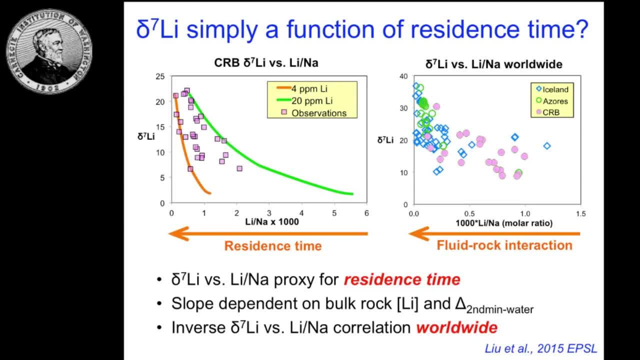 of the basalt we put in. So it seems to work out pretty well. with increasing residence time We have higher fractionation And also we tried to compile some data from literature where we observed the Atlantic rivers and also rivers from the Azores. 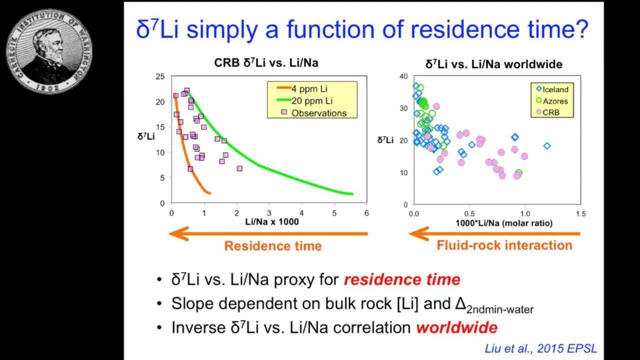 where people only see the weather of basalt right, And this seemed to have the similar trend in terms of lithium sodium ratio versus delta-lithium. So we would like to argue that the residence time controls the delta-lithium and lithium-sodium ratio behavior. 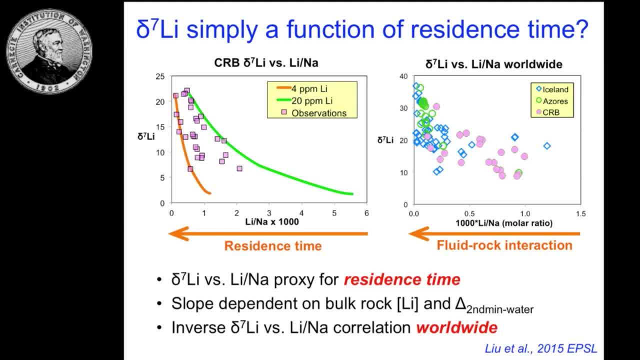 It's reflecting fundamentally the residence time. In another word, it's fluid-rock interaction: how long the rock has been influenced by the water, right? So these correlations seem to be a worldwide effect, not only small study. What? Why do the pink points look different? 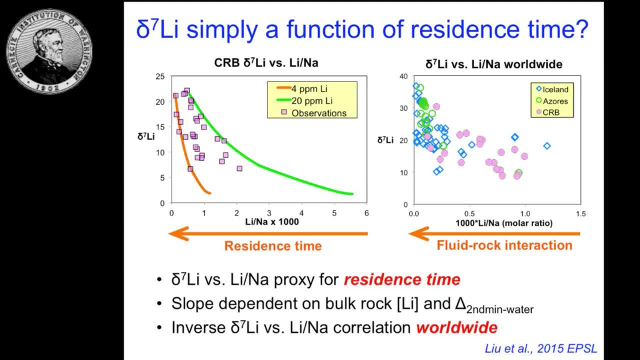 from the blue points? Oh, because the I think, because the- Let me see, I think because the scale is different. So there were some over there. It didn't show over there. Okay, Right, Right. And also maybe this: 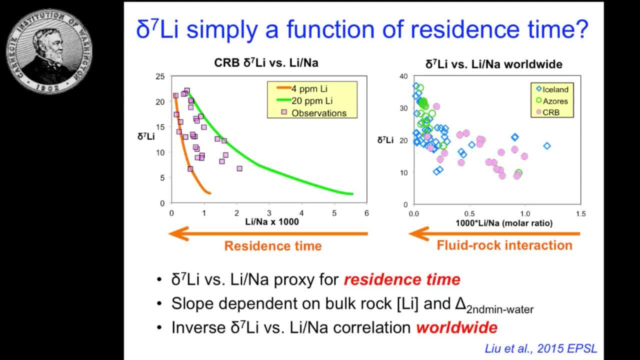 I think this one. I already got rid of the groundwaters. This one has the groundwaters. Yeah, I think. Yeah, Too many colors, Sorry, Okay. So the bottom line is: I just wanted to show you what controls delta-lithium in rivers. 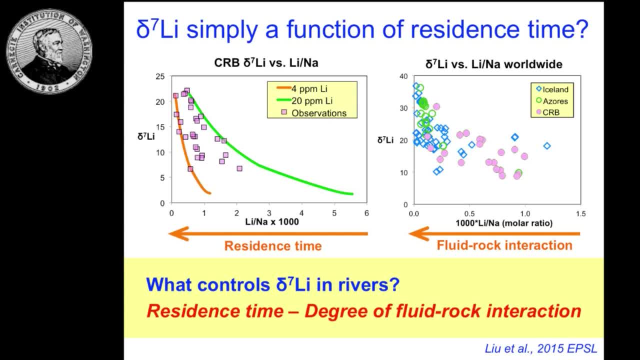 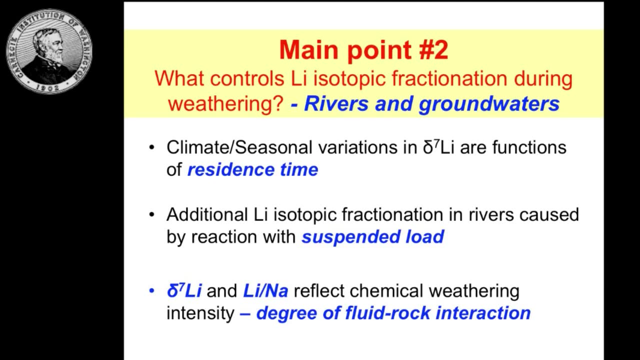 with lithium is the residence time, So it's not the fractionation factors between two different minerals versus the. you know the water or weathering regime argument, So Anyway, So this is another way to emphasize, I guess, the seasonal variation also. we saw 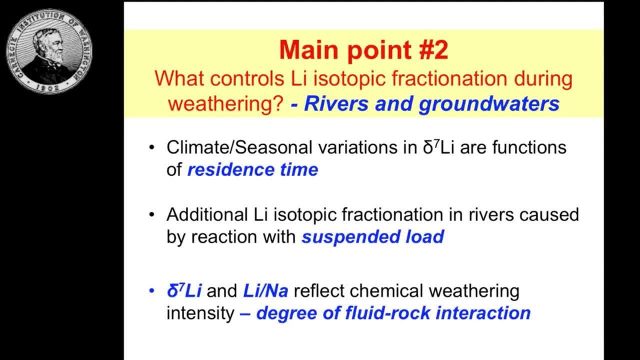 is another good example why the residence time is important. Remember we I showed you the. The delta-lithium in the summer is actually have higher compared to the, Compared to the winter. right The summer because the western has a lot of. 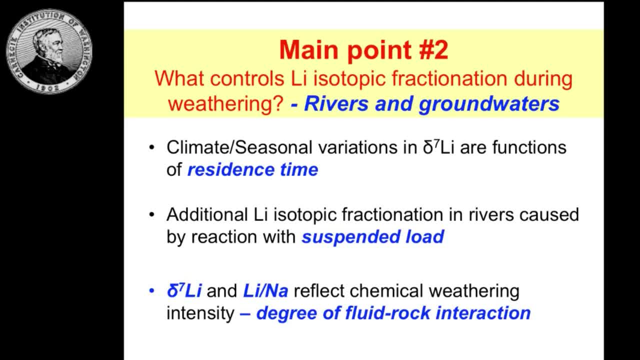 Western or the Cascade. I mean the western has a lot of precipitation and then you have more residence time between the water and also the weathering profile of the soil. That's why you could- You could- have heavier delta-lithium. 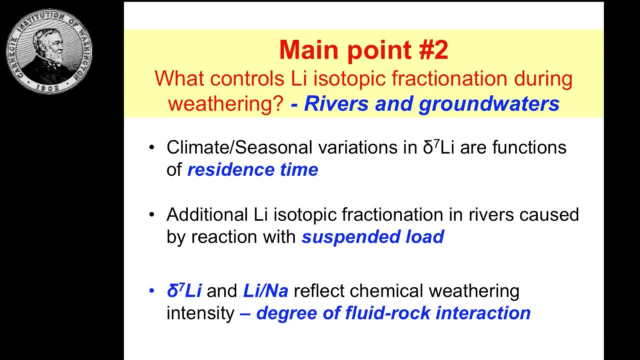 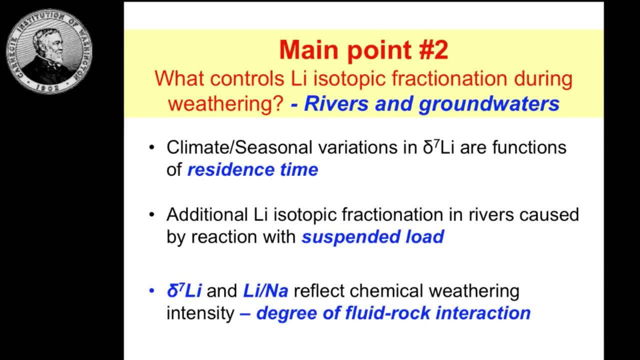 And also the other important thing is there is an additional lithium fractionation in the rivers because we assume there is additional reaction between the suspended load and also the water right. That's why you have fresh kind of small rock chips or small particles in the rivers. 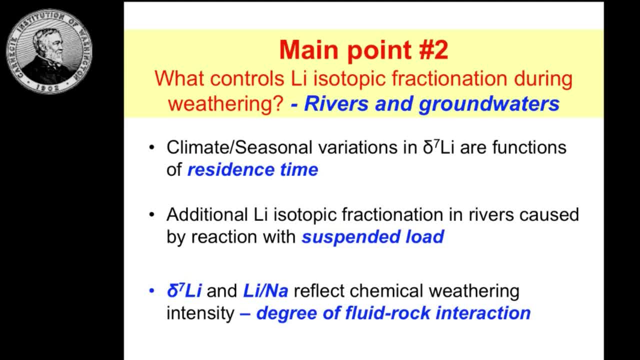 and then they keep, Keep reacting with water as they transfer along. So that's why we got additional lithium fractionation in rivers. Okay, Thank you. Okay, Okay. So here is the. that's actually what's observed in nature as well. 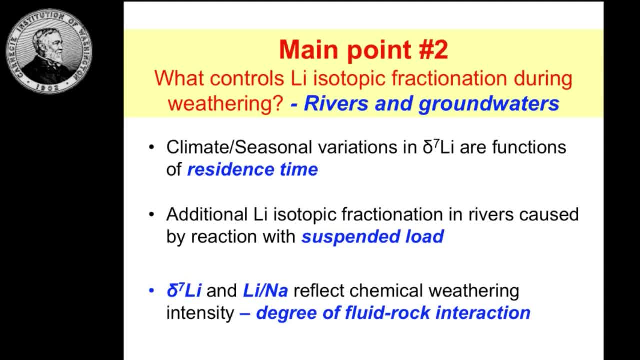 so we would like to propose there's possibly a good proxy for the delta lithium versus the lithium sodium. they're actually reflecting the degree of the three rock interaction, so by plotting where on the line we can try to figure out how much of the weathering is going on. 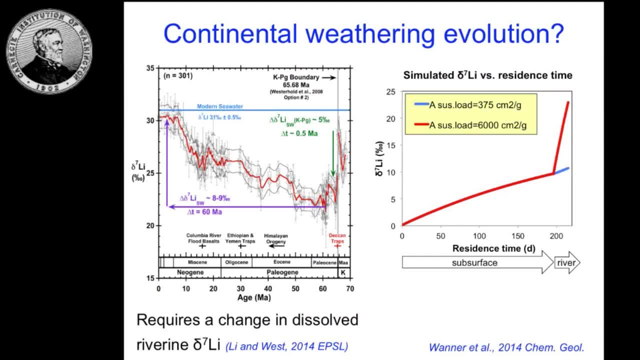 right, so, oh okay. so one more thing we want to, as I originally showed you this very intriguing study where we see an increase of delta lithium through the celluloid. so now we would like to go back to try to explain a little bit more, because we know that this increase has to. 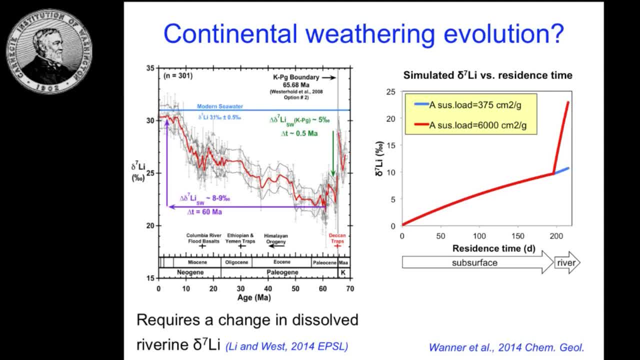 require a change in dissolved river in delta lithium. so we are kind of ignoring the hydrothermal input change and also the orthogenic clays output, right? so because this study showed we need to have a rivering change to have this dramatic increase in terms of marine delta lithium values. 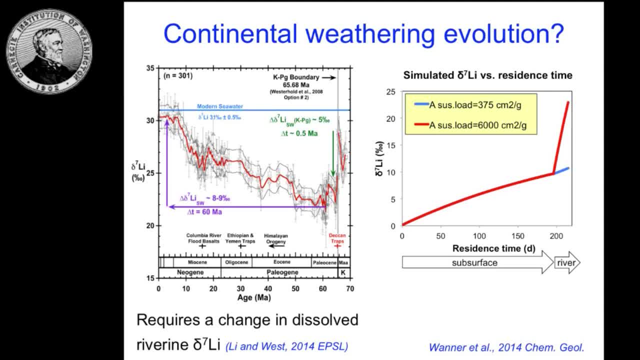 so, collaborating with Chris Warner, we have done a global scale simulation where we look at the weathering from the granite, because that's the average composition of the African crust. so this one- I just show you one simulation result that may be useful for explaining why we have this large increase. 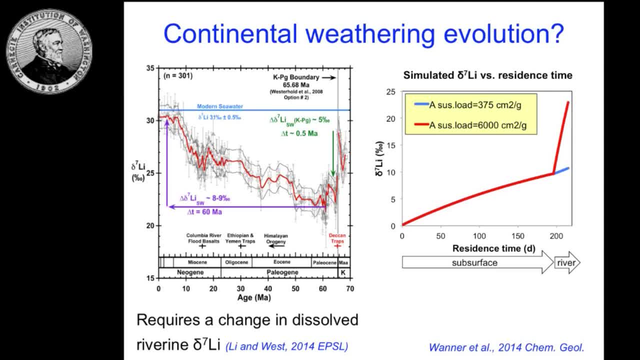 because if we do a relatively small suspended load, so this part is also the river and that's a large suspended load. so if we have increased the weathering intensity, meaning we have a lot of fresh materials to weather, we could generate a much larger delta lithium. so this actually goes with the rise of the Himalayas. 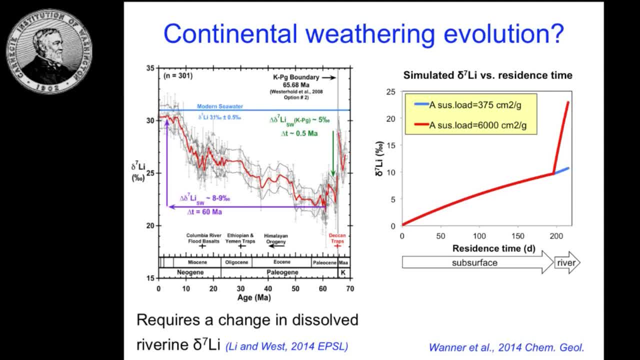 because there is a mountain building. mountain uplift can cause more erosion, which generated a higher suspended material in the rivers. we can have higher delta lithium. so that's still one of the reasons to explain so. the tectonic aphidus caused an increased weathering. to explain the mizora and folic diagram here. 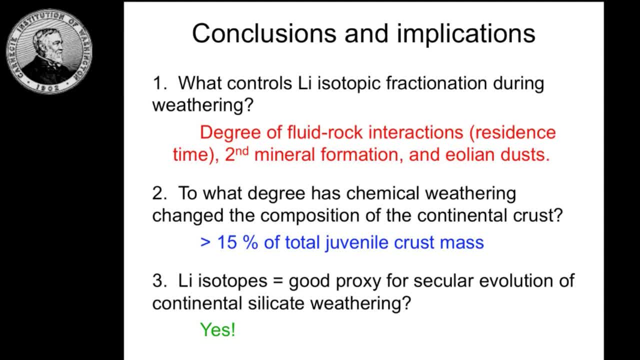 so, to conclude, I hope I convinced you that the degree of fluid rock interaction, or the residence time, is very important in terms of controlling the isotopic behavior, as well as secondary mineral formation and aeolian dust, because the weathering is an open and dynamic system. it's not a closed system. 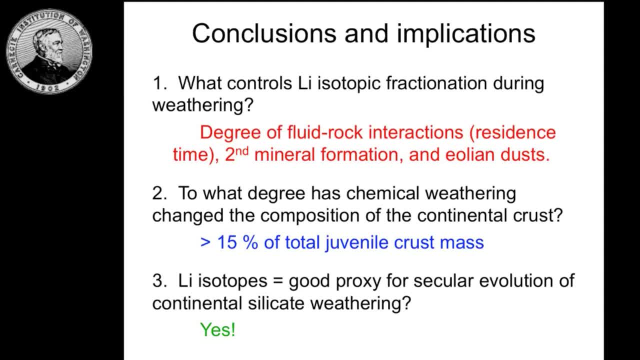 so you need to be always careful with additional dust and this one I didn't explore, but we already showed there is at least 50% of the total juvenile crust mass has been lost due to weathering. that's like a cumulative effect. it's over the history. 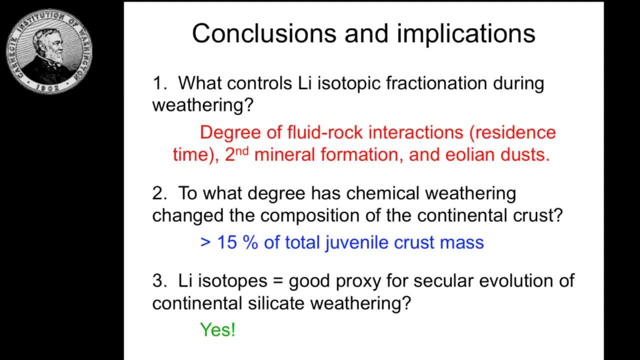 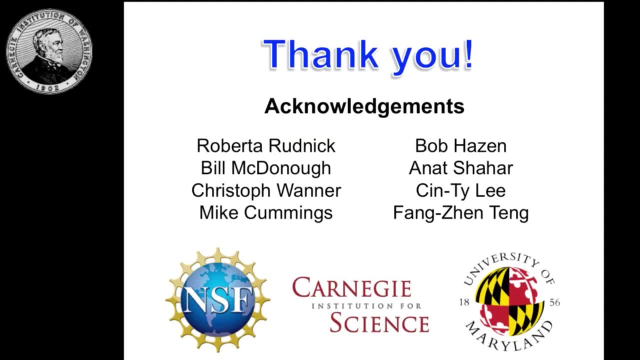 the earth's history, so it doesn't have a flux component. so, and also- yes, I hope by now you are still awake- and also, lithium is a good proxy for secular evolution of the continental silicate weathering. okay, with that, I would like to thank all my collaborators. 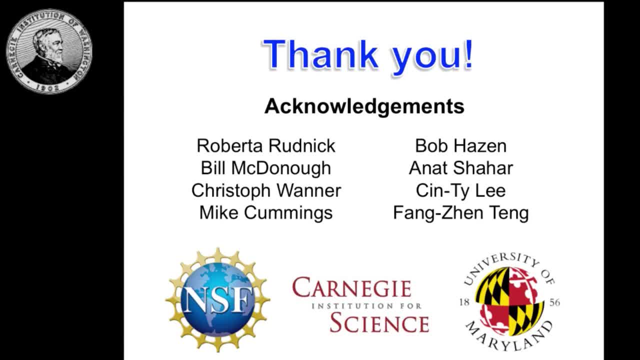 in the lithium work, as well as my mentors in the geophysical lab for the postdoc fellowship, Bob and Art and others for inspiring, for doing this part of the study, and I'm grateful for all of you to come in a nice summer day. okay, thank you. 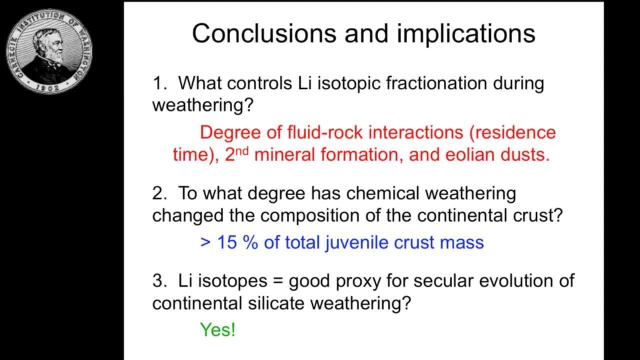 all right, we have time for a few questions, so a very nice talk. I was going to ask you about the river, but you explained that. so it's a combination of the mechanical combined with the chemical. so another question I would ask is: carbonaceous chondrites have been very extensively altered. 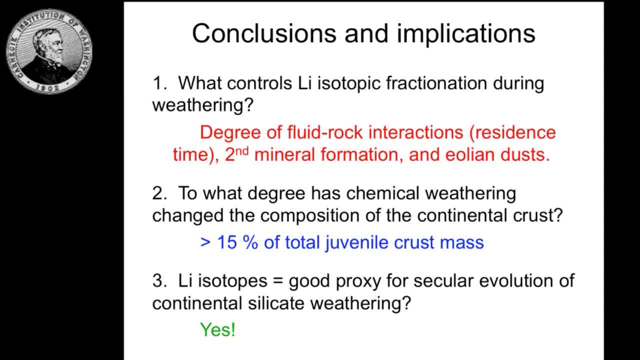 and the question has always been: how do you measure how expensive, because you just have residue in the back. is there any way you can use lithium isophenides to make a specimen about sort of what the water-rock ratio might have been during the parent-body evolution of a? 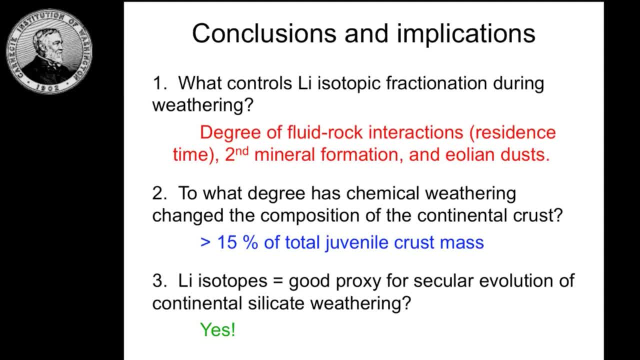 now say C1 type chondrite. right, yeah, that's a. yeah, that's a great question, but depending on the operation temperature though. so if this was higher temperature, then the fractionation is not pronounced. so I don't know what's the could be the it's more hydrothermal temperature. 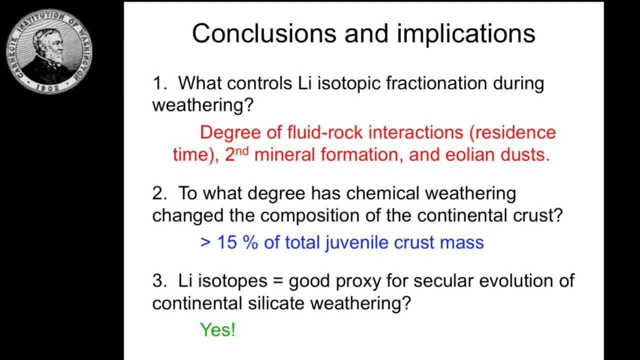 or surface temperature, that's. that's another question. but if it's hydrothermal temperature, then the fractionation is more small, as you know that it's negative correlated with temperature. that's why we- I swear I- switched my study to low temperature for lithium, because we have C-bake fractionation. 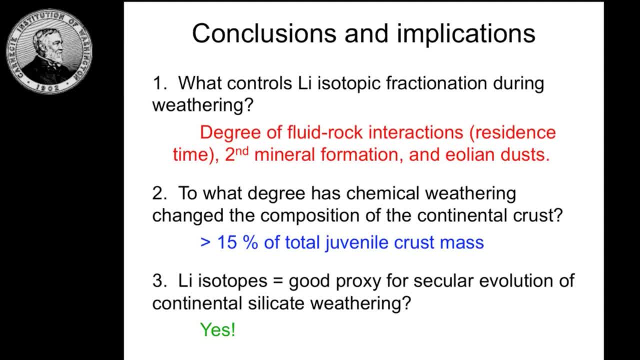 but that's a good point if you think about that. I have two kinds of questions. one has to do with the chemical weathering. did you measure both the dissolved load and the suspended load in the same samples- right yeah? of lithium isotopes and concentrations? right yeah? so we measured where we can. 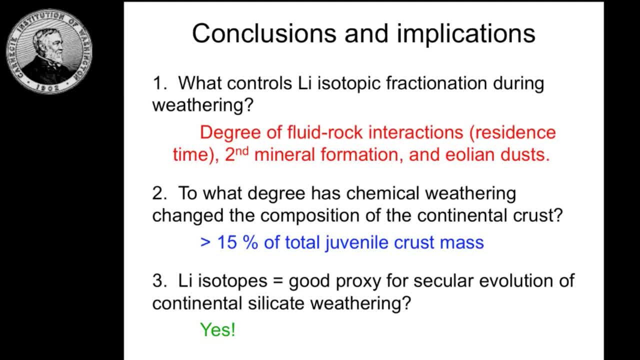 because it's the first time to do this. you know the rivers as I show you. probably it's not already clear, but those are really pristine rivers, those are pristine streams actually. so those are having really low suspended components. so we filter them, we use a filter on site. 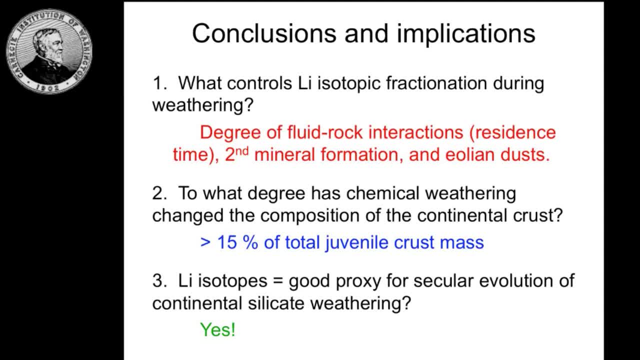 using a peristaltic pump to filter the material. so we do have a filter size of 0.2 micron. so anything lower than that is we classify as dissolved. and then there are some particles on the filter. I dissolve them and then analyze the suspension. 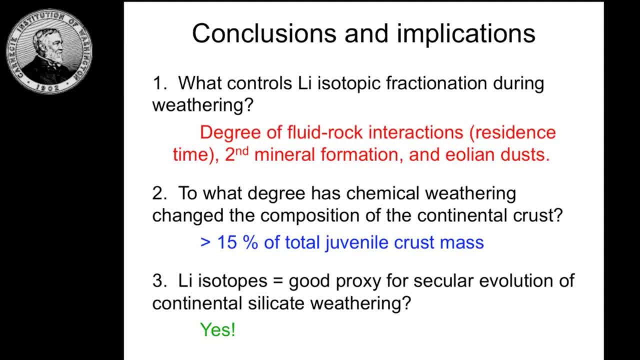 and the suspended part, so the suspended part actually having slightly lower value. did you show those data? I didn't show the suspended part. could you make statements about the suspended load? but I don't remember seeing any suspended load data. right, yeah, that's a good point because there is only half of them. 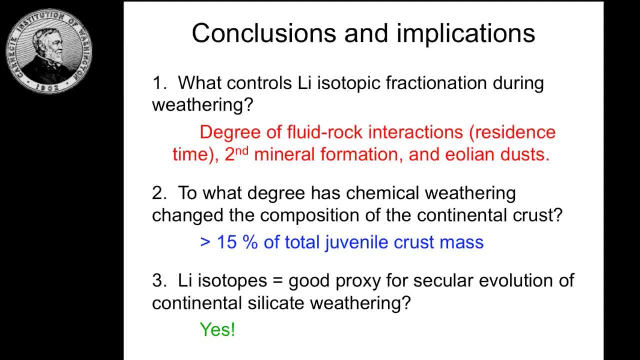 I kind of got the suspended load because it's pretty clear river, there's not much of suspended load so we run the filter for a long time, but still there's. so a type of question. I was wondering: if fluid rock interactions are important at ambient temperatures, would they be important at high temperatures? 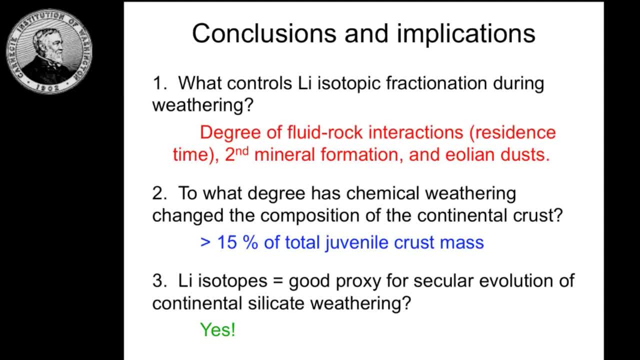 does metamorphism matter? does hydrothermal alteration matter, particularly if you're interested in this composition of how the composition of the continental crust has changed over time? you know studying fresh basalts, so have you thought about metamorphic processes and hydrothermal processes? yeah, so a metamorphism is important. 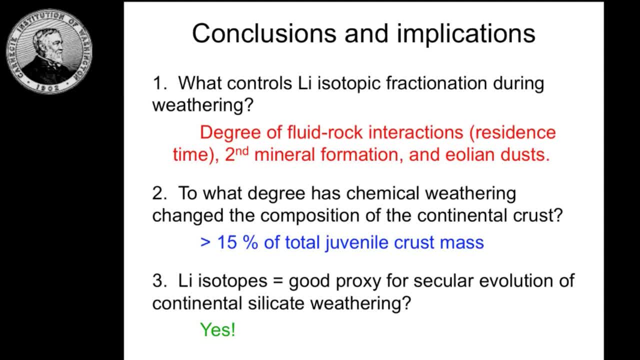 in terms of lithium content, not much in the isotopic composition. so people already did the study from the Green Schist metamorphism, very low metamorphism to like granulite phases metamorphism. so the delta lithium actually in a rock doesn't change. so because it's a high temperature fractionation.